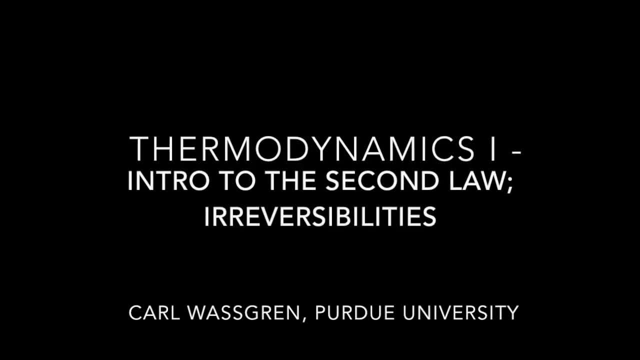 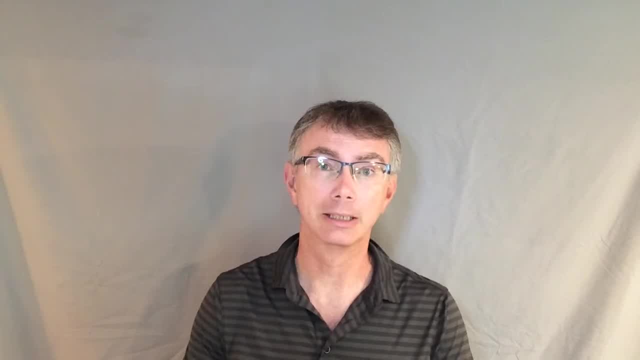 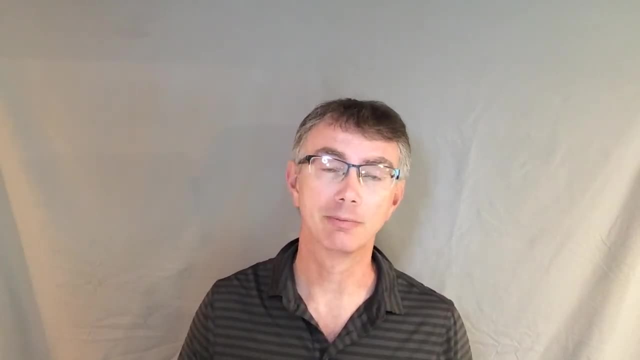 Well, welcome to this video lecture on the introduction to the second law of thermodynamics and as well as a discussion on irreversibilities. In prior video lectures we focused primarily on the first law of thermodynamics and conservation of mass, two very important relations. They're. 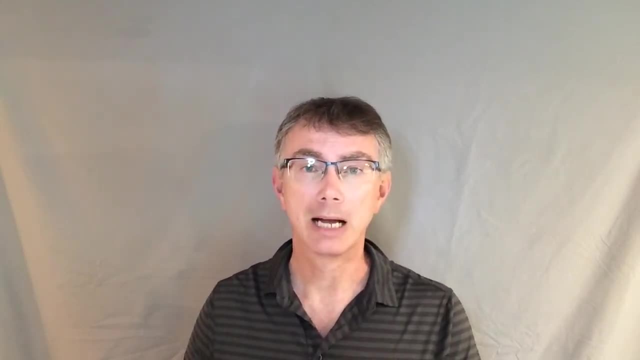 used all the time in thermal fluid systems. We're now going to move into a different topic, and that's the second law of thermodynamics. It's not used quite as often as the first law, but it is used frequently to determine whether a process can or can't occur. And 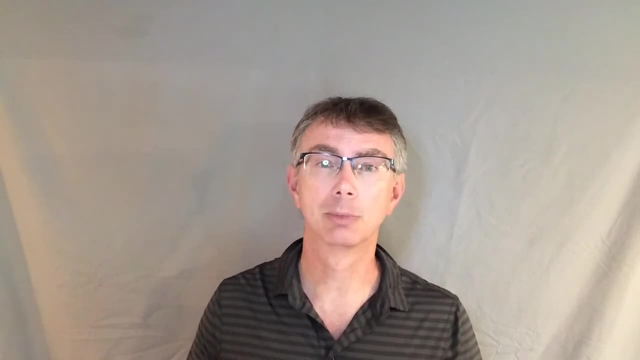 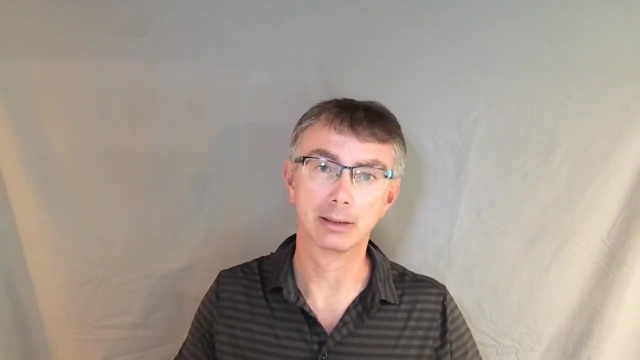 it can also be used to establish maximum limits of performance so that we can define efficiencies that we can then use to investigate the effectiveness of real operations. So we can establish a maximum limit by using the second law and then compare a real process to that ideal. 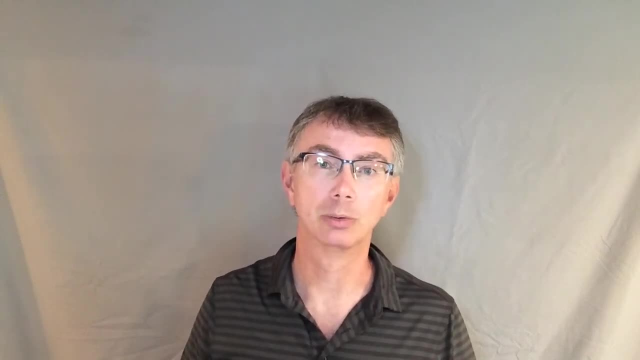 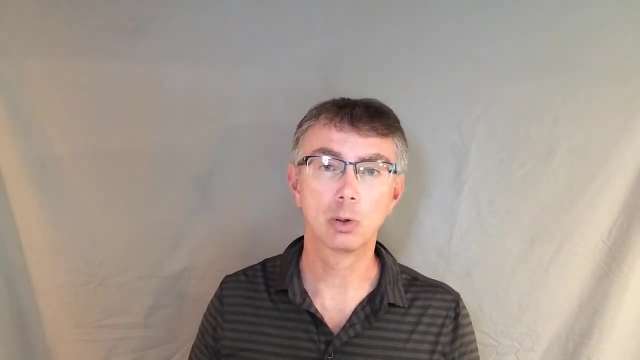 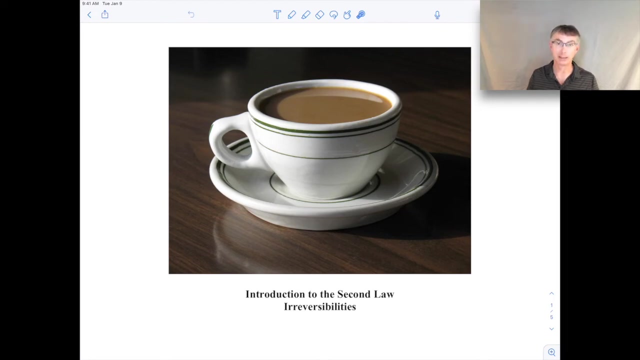 operation. So that's really where we get a lot of use out of the second law. So go ahead and take a look at your screen. You'll see a picture of a coffee cup, And the reason I showed this picture is because often people add cream to the coffee, like in this particular cup. 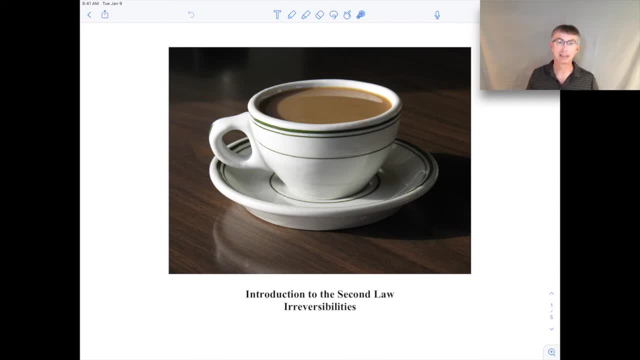 of coffee And, of course, when you add cream to the coffee, it mixes in and becomes well distributed within the coffee itself. That mixing process is an irreversible process. It's one of many different irreversible processes, But an irreversible process is one that doesn't. 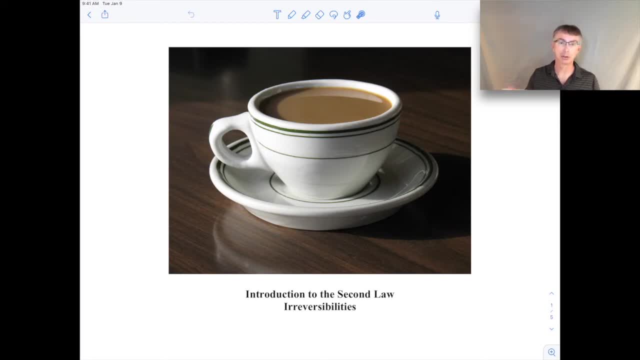 naturally go back to its original state. So if you put the cream in the coffee, it mixes distributes everywhere, but you never see the reverse happening, where the mixed cream suddenly comes together back into a single clump of cream. right, That just never happens. 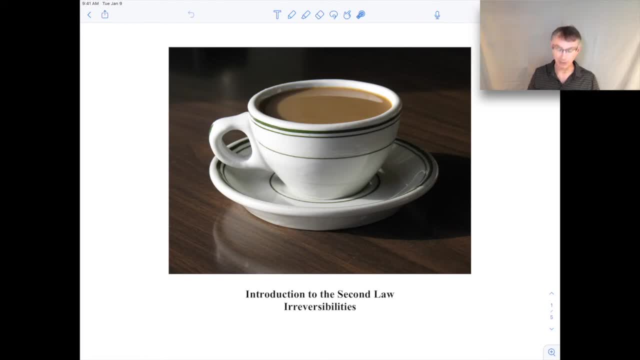 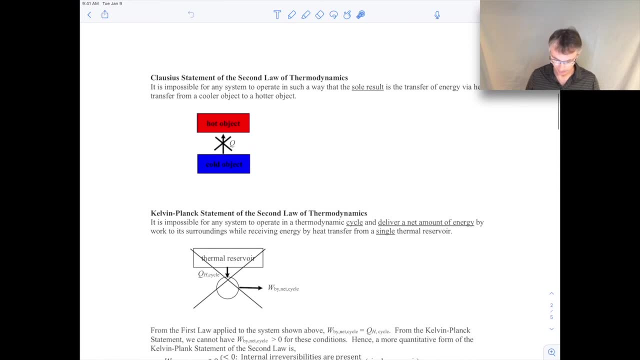 It's irreversible when you mix it in there, And so this is a—mixing is one example of an irreversible process. OK, so the first thing that we're going to do is talk about two fundamental statements for the second law of thermodynamics. They're both equivalent to one another. They look 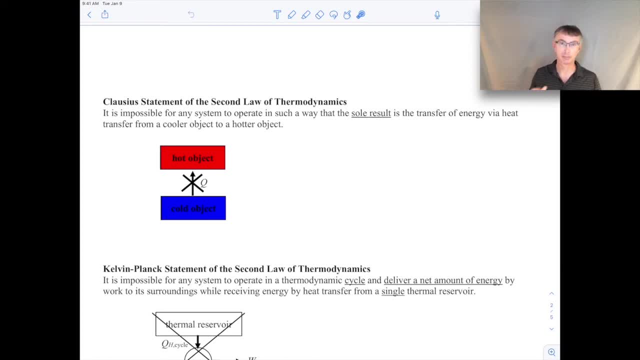 different, but you can demonstrate that they're actually equivalent through some thought experiments. But they're very basic statements. The first one is the Clausius Statement of the Second Law of Thermodynamics, given right here, And it states that it's impossible for any system 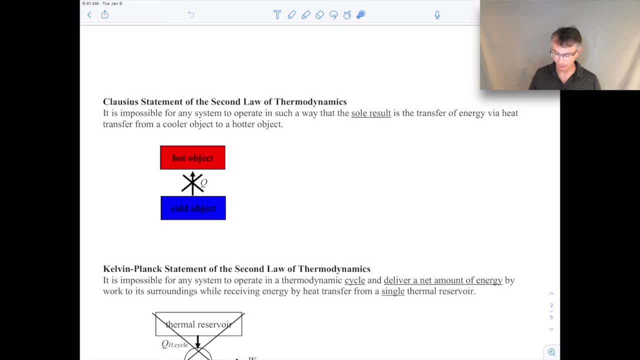 to operate in such a way that the sole result is the transfer of energy via heat to the atom. the second law of thermodynamics given right here, And it states that it's impossible for any system to operate in such a way that the sole result is the transfer of energy. 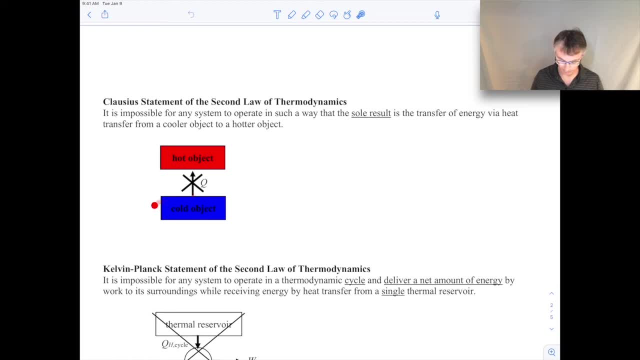 via heat to the atom, And it states that it would be possible to follow the same process by developing an eternal process in both equations. So what we're going to do is go ahead and heat transfer from a cooler object to a hotter object, So we have a cold object. 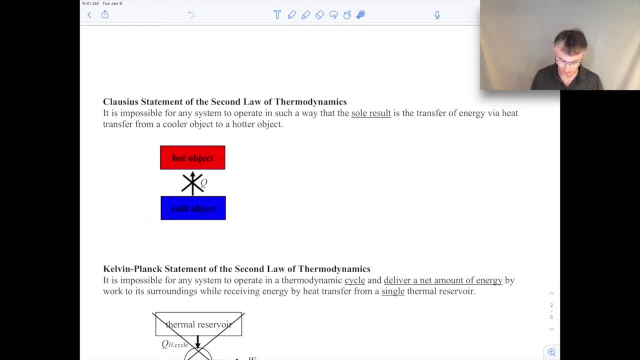 here. so a lower temperature hot object up here, and we just never see energy being transferred from the cold object to the hot object via heat transfer. It just never occurs. And based on that empirical observation we form this statement of the second law of thermodynamics that we just can't expect. 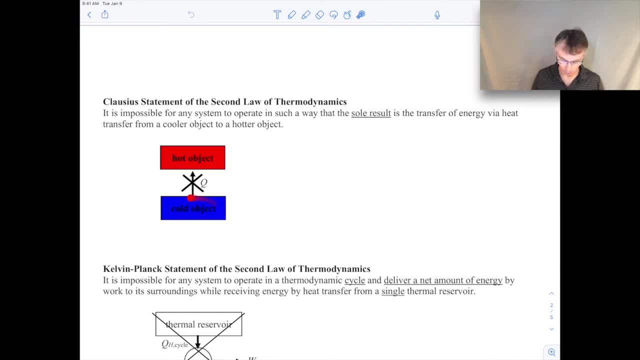 in nature, heat or energy to be transferred from a cold object to a hot object, just spontaneously occurring. You can do it if you put some work into the system. but if you don't do any work on it it's just never going to. 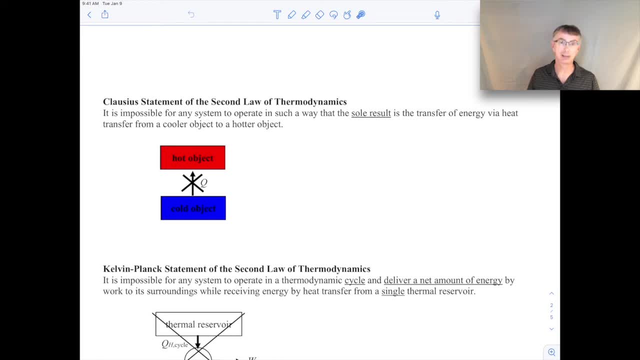 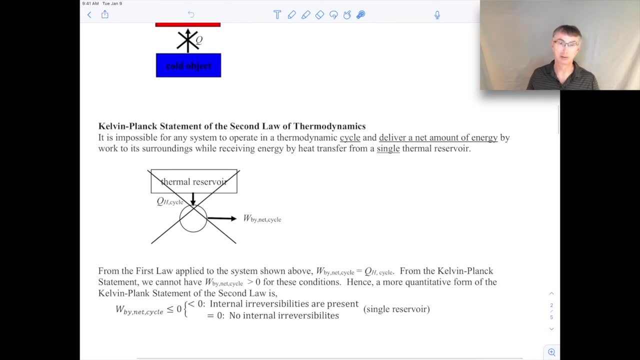 spontaneously occur. So that's the Clausius statement of the second law of thermodynamics. Now the next form of the second law of thermodynamics is called the Kelvin-Planck statement, And again I'll show a little bit later that these are actually equivalent statements. 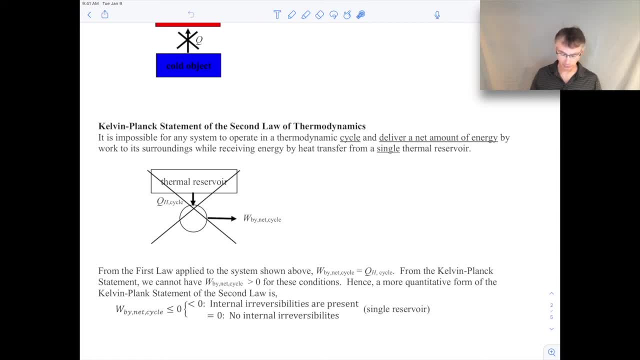 They just look very different initially. So the Kelvin-Planck statement is that it's impossible for any system to operate in a thermodynamic cycle. the cycle here is important- and deliver a net amount of energy by work to its surroundings, while receiving energy by heat transfer from a single. 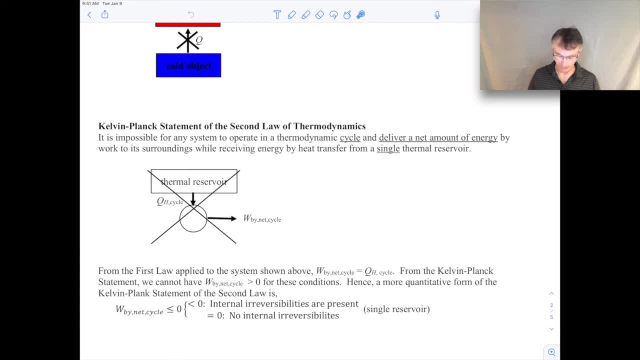 thermal reservoir. The single is an important term here as well. So it corresponds to this picture where we have a thermal reservoir, like a hot thermal reservoir, and we can't have heat transfer into our system. So this would be our system operating on a cycle. We can't have just 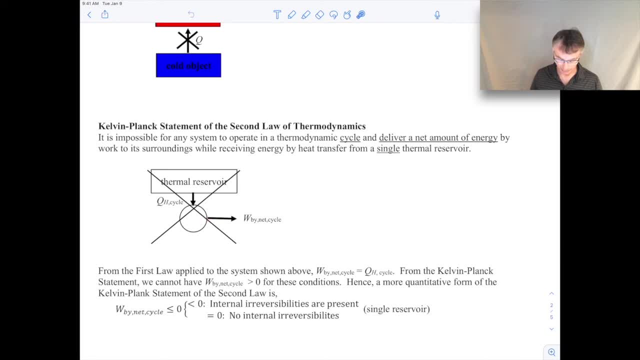 heat transfer coming into that thermal reservoir and then going out to generate some work. We can't have it. There's going to have to be some heat coming out of the system into a cold reservoir, as we'll see a bit later, But just going from a single. 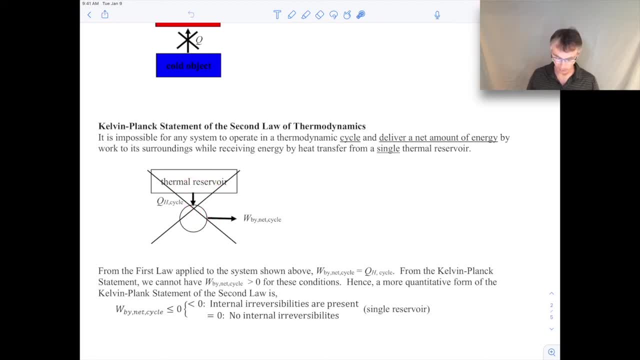 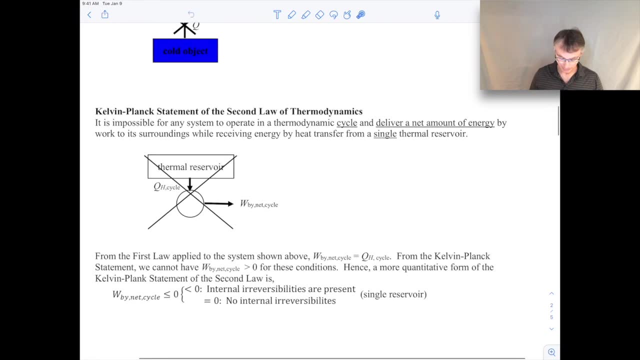 thermal reservoir into our system and then getting work out of it is just not possible. So that's another form of the second law statement And if you apply the first law to this system shown here, so this is our system and you apply the first law to. 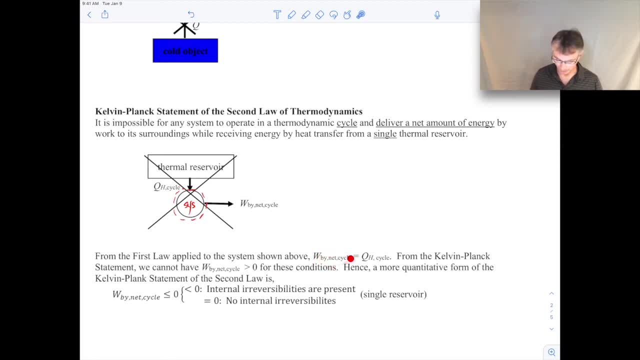 that system. you'd see that the work done by the system, the network done by the system over the cycle is equal to the heat energy coming in from that hot reservoir over the cycle. So you get this expression. Since it's a cycle, there's no change in total energy over the cycle and 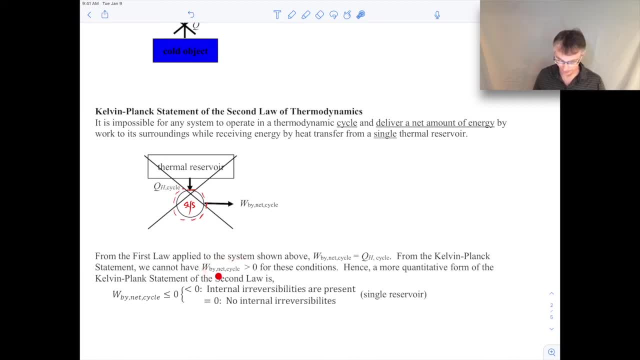 then from the kelvin-plank statement we say that we can't have that work being positive for these conditions, right, that that would correspond to this picture in the kelvin-plank statement says it's not possible to do that, So a. 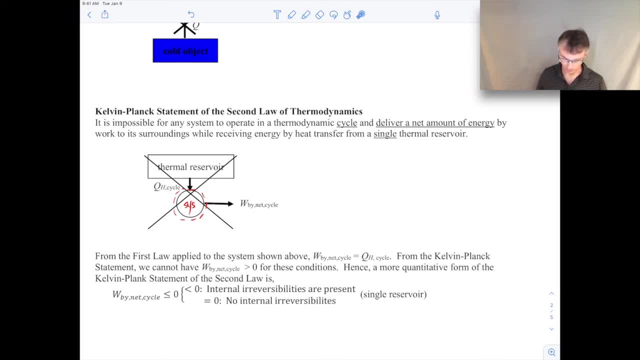 more quantitative way to write that kelvin-plank statement is to: since it can't be positive, it can only be less than or equal to 0 over that cycle. So we know that it can't be positive. it has to be less than or equal. 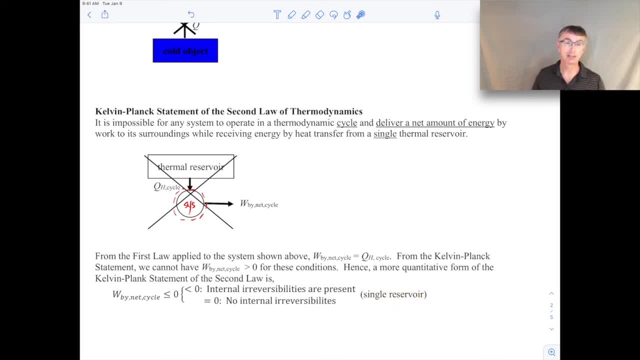 if you're dealing with a single reservoir, and one of the things that we'll find a bit later is that the equal sign only holds if there's no internal irreversibilities. So we'll talk more about irreversibilities in a little bit, but an internal irreversibility- internal just means internal to. 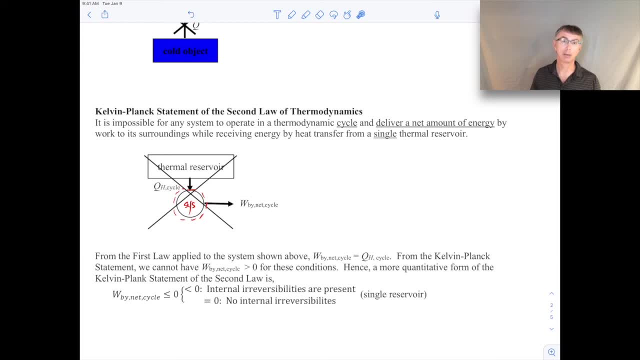 the system and an irreversibility is something that just doesn't go back to its original state, like the mixing I talked about a moment ago. So if there are no internal irreversibilities, then you use the equal sign here, So the network, if you do this kind of single thermal reservoir. 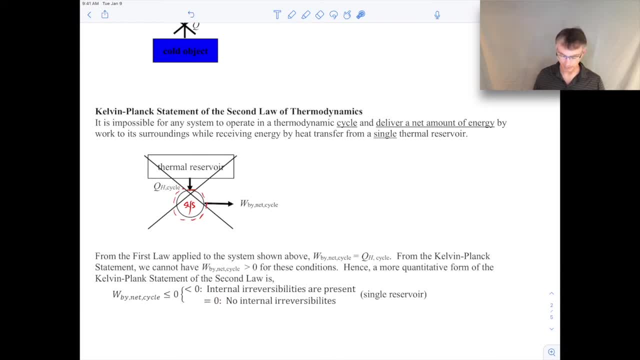 heat coming in. at best it's going to be zero work that you're going to get out, and then if there are internal irreversibilities that are present, then it'll be negative. So you'd actually have to be putting work in to that if there are some internal irreversibilities going on over the 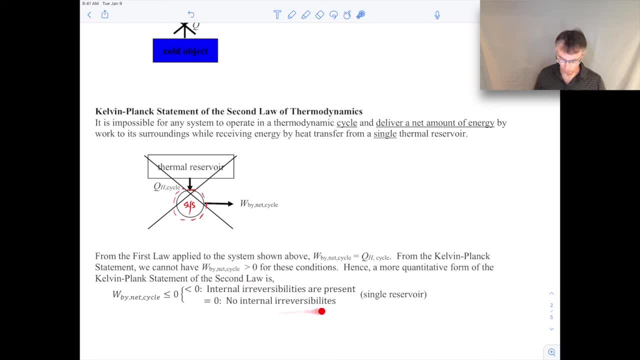 cycle. So this sort of more quantitative form of the Calvin-Planck statement just follows naturally from this picture. We're just saying that we can't have a positive work out over the cycle, which means that it could be less than or. 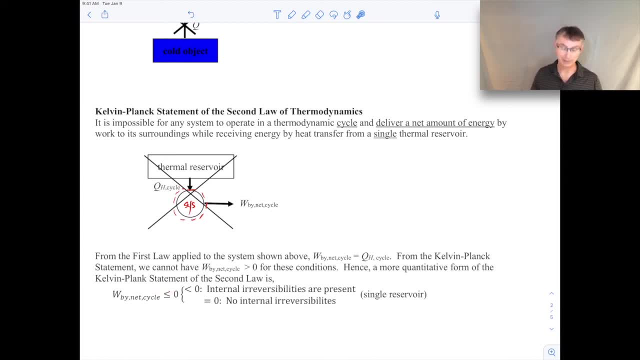 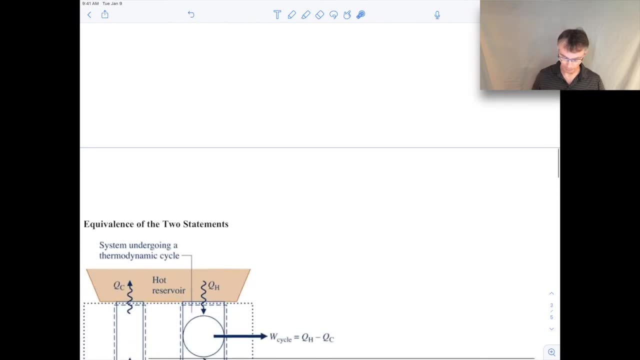 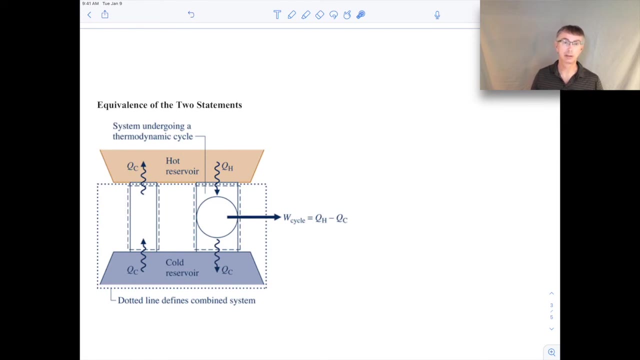 equal to zero, and then the less than or equal depend on whether there are some internal irreversibilities or not. Okay, now let me just demonstrate to you that the two statements are equivalent to one another with the thought experiment shown in the picture. 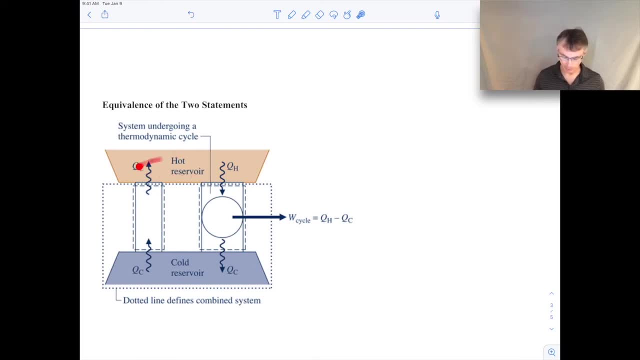 So what we have is a hot reservoir up here and a cold reservoir here. We've talked about what reservoirs are. They're basically hot reservoirs, just at a high temperature, and it doesn't matter how much energy we take out of it, It always stays the same temperature. It's infinite in size, Same. 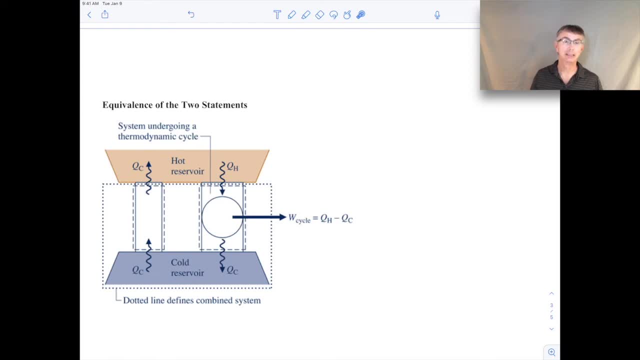 sort of thing with a cold reservoir. It stays at the same temperature. It's a lower temperature, Infinite in size. It doesn't matter how much energy you put into it, It always stays the same temperature. And then we have a couple of systems here. So we have a system, you know, kind of a. 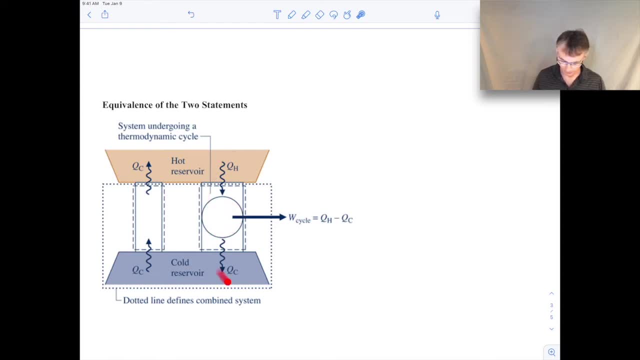 traditional system and then we have a system that's a little bit more complex. So we have a traditional system here. So the picture that we have on this side looks kind of like something we've talked about before when we first started talking about cycles. We've got some energy. 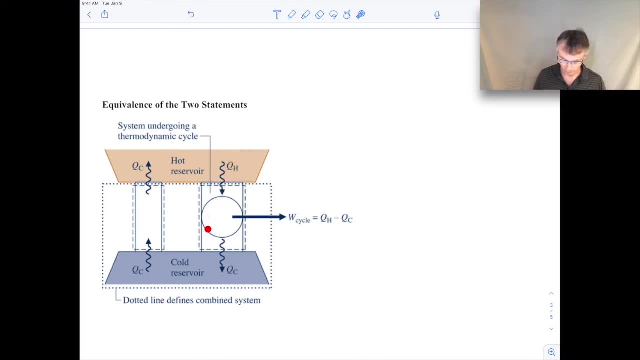 coming in from the hot reservoir- We'll call it QH- into our system. We're pulling some work out of it over the cycle. So this is all operating on a cycle. So from the first law the work that we get out would be the QH minus QC. QC is the thermal energy we're putting into the system. 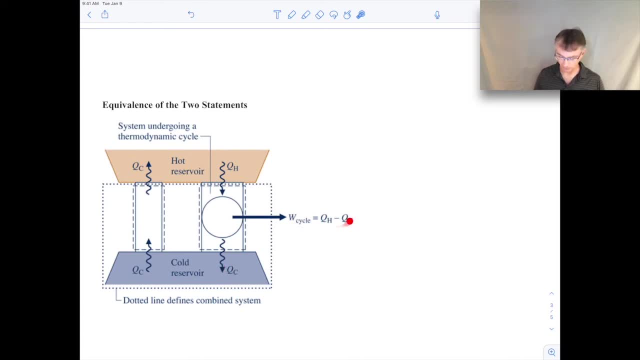 So this is the thermal energy we're putting into the cold reservoir QC. So this comes from the first law. So so far that looks pretty good. And then what we're going to do in our thought experiment is we're going to have? we're going to take that same energy that we put into the 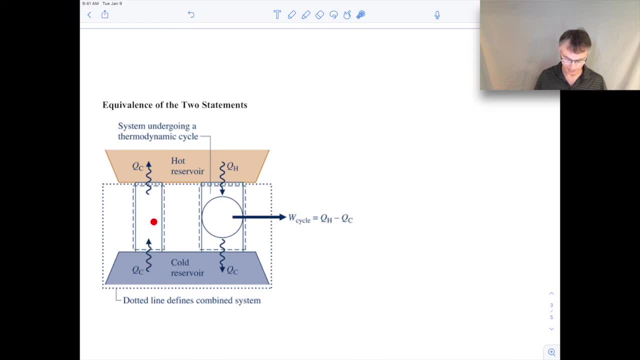 cold reservoir, We're going to just take it right back out and spontaneously have it move up into the hot reservoir. So this QC moves just straight up into the hot reservoir. So we're taking some energy and spontaneously moving it from a cold temperature to a hot reservoir. 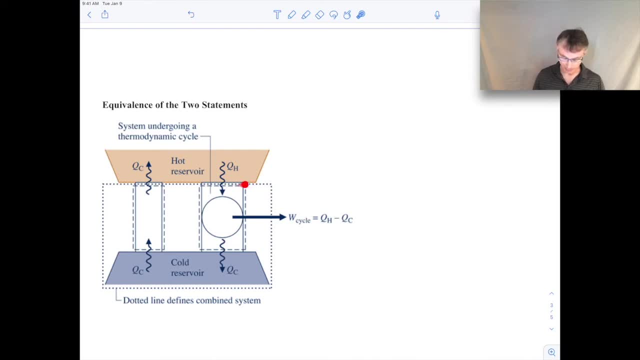 Now, if we do that and then we draw a dashed line around this whole system, then that picture will look like the Calvin Planck picture. It'll look like this. Let me sketch it over here: So we have our hot reservoir, We have our system, And then we're going to put some heat into it. The heat. 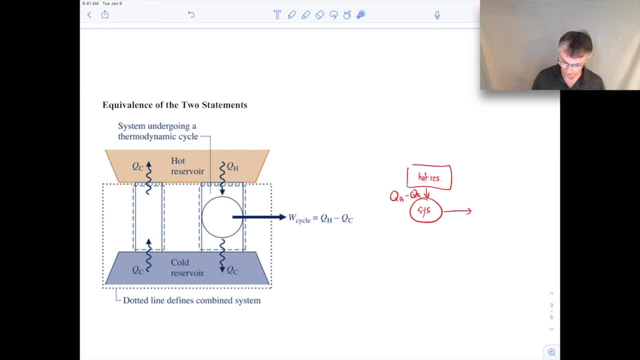 that would go into it would be the QH minus the QC. You can see that the QH minus the QC. here And then we would get some work done out of it by the cycle And you'll notice that we're not discharging anything in the cold reservoir because we're putting some energy into. 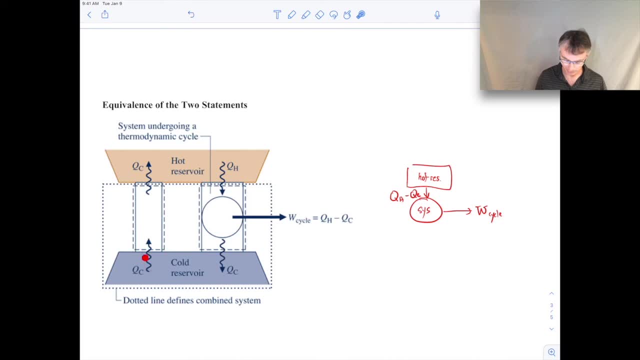 the cold reservoir here, cold reservoir here, and then we're removing that same energy here. So the net amount of energy that we put into the cold reservoir is zero. So you can see that this picture, we know, is the picture that we just talked about in the Calvin Planck statement of 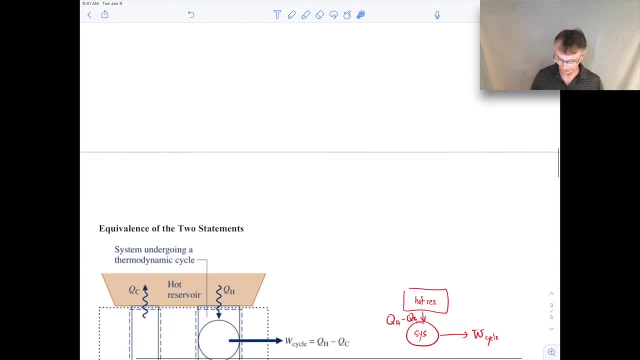 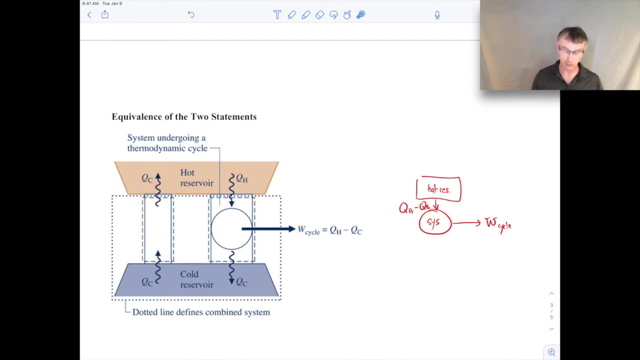 the second law looks just like that picture. So we know that clearly this part of the original picture that is a violation of the Clausius statement of the second law, where we can't just spontaneously move energy from a cold reservoir to a hot reservoir. That would violate the Clausius. 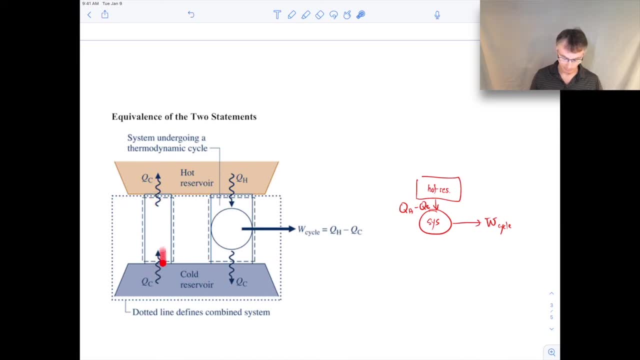 statement of the second law. If we can't have that, then we're not going to be able to have this picture either. If we have that situation where we violate the Clausius statement of the second law, it means we're also going to violate the Calvin Planck statement of the second law, because this picture corresponds. 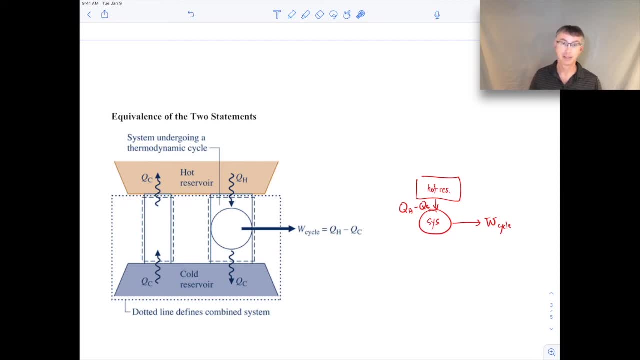 to this system in the dotted line here. Similarly, if we say that this can't occur- this is the Calvin Planck statement- if we say that that's not possible, of course we could make that system. we could just expand it out into this kind of picture. and if that's not going to happen, certainly this: 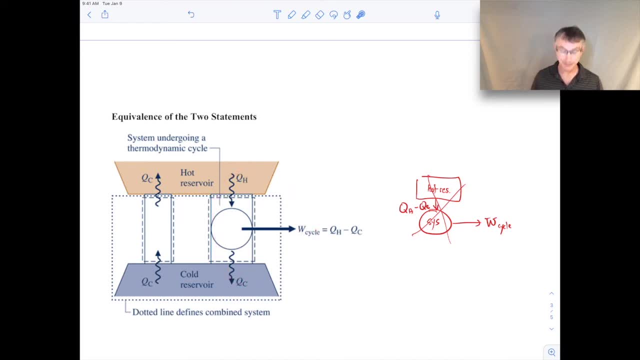 one can happen. There's no issue with this. This picture is fine. It doesn't violate the Calvin Planck statement, because we're not only bringing energy in here, but we're offloading some energy too. We have two thermal reservoirs, not just one. so it's okay, This one's okay, but if this is not okay over here, then this: 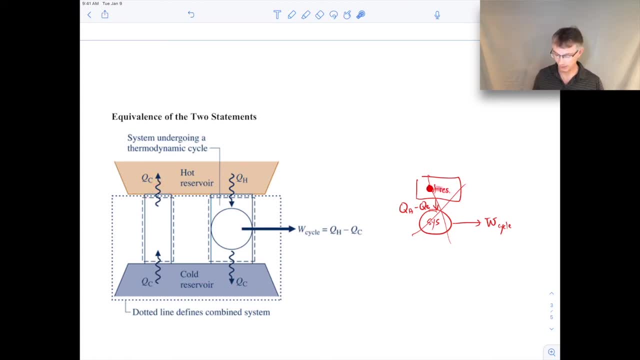 part must be incorrect. So if we have a violation of the Calvin Planck statement of the second law, then that means that we're also violating the Clausius statement of the second law. So this is the demonstrated equivalence between the two. You can draw a more complex system that looks like this, where, if you violate one of the second laws, 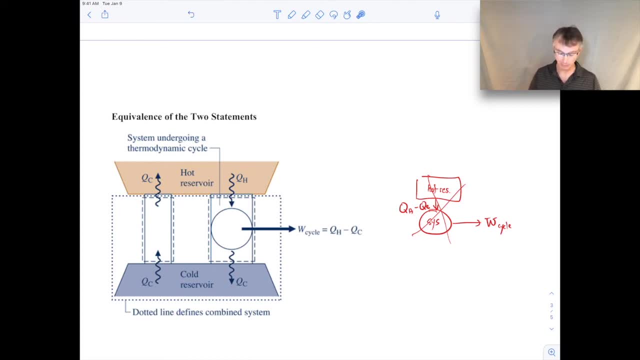 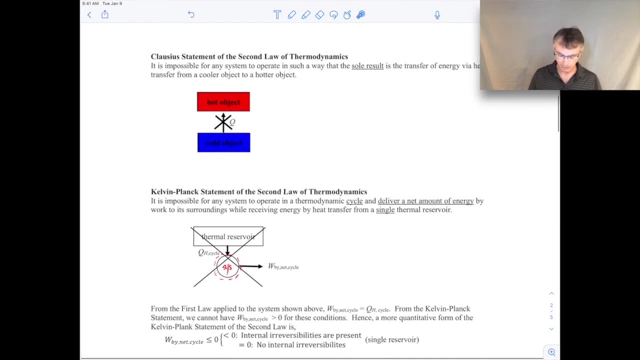 you're going to violate the other, and vice versa. So that's what we mean by the equivalence of the two statements. So what I find interesting about all this is, from these simple statements of the second law- the Clausius statement and the Calvin Planck statement- you'll see that we're going to end up. 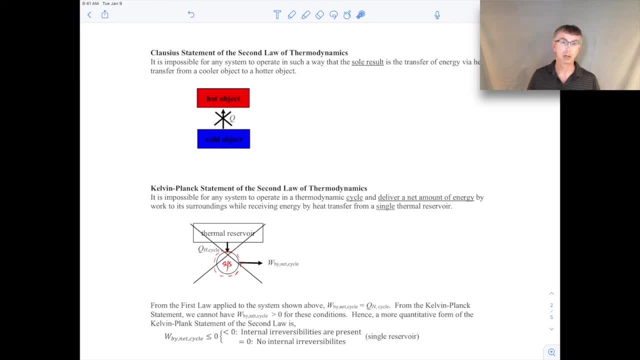 ultimately defining this property known as entropy from all of this. They'll take a couple of steps to get there, but we'll define this property of entropy and then use that property of entropy to actually do some numerical calculations. And I think that's just kind of a neat thing that we go from a very kind of general statement. 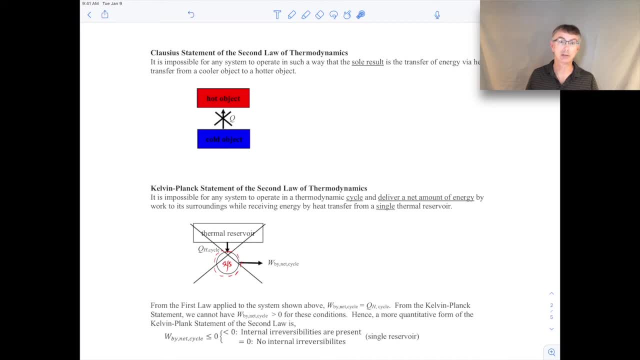 these two general statements just based on observations made in nature, and from those general statements we make it more quantitative and then define this property entropy that we can use to actually do real calculations, And I think that's just very interesting and neat. 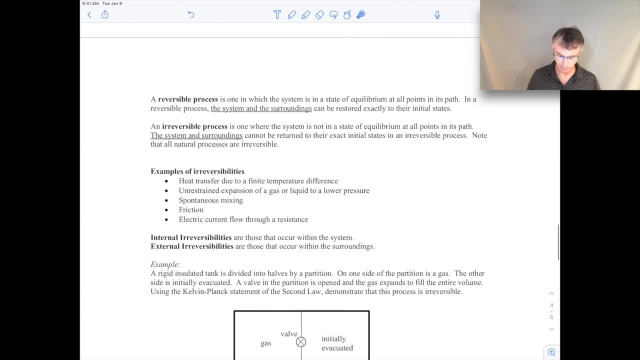 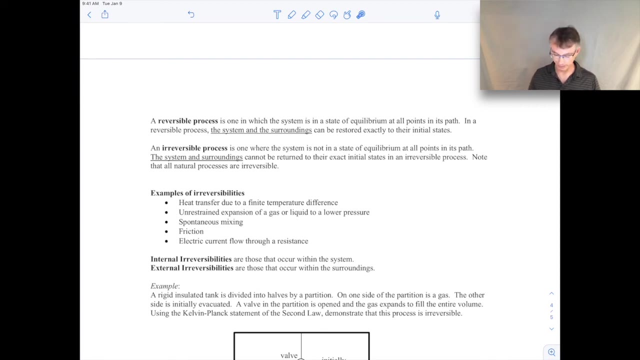 Okay, Let's talk a bit about reversible and irreversible processes, because that's something that I started with with the coffee cream in the coffee example. So, first of all, a reversible process is one in which the system is in a state of equilibrium at all points in its path. 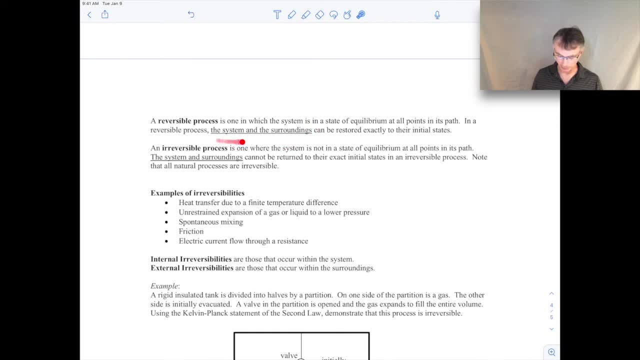 In a reversible process, the system and the surroundings can be restored exactly to their initial states. It's reversible meaning that when we go in that path from- you know- state 1 to state 2, we could go back from state 2 to state 1 and both the system and the surroundings come exactly. 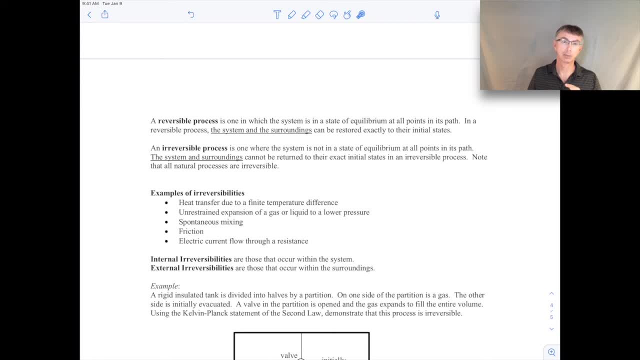 back to where they originally were Right. so it's important that the system and surroundings are returned back to their original state. so states So it's reversible. You can always get back to where you started from Now. an irreversible process is the opposite of that. it's one where the system is not in a state of equilibrium at all points in its path and the system is not reversing. 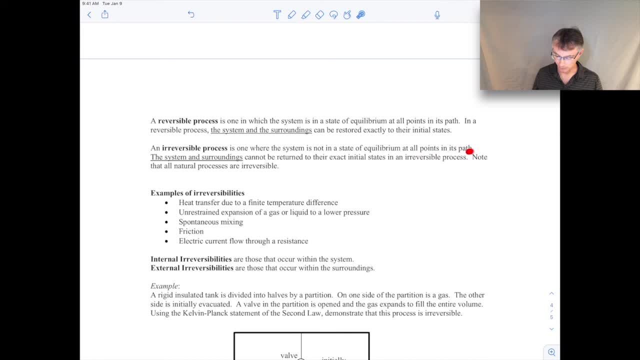 '' aza e of random, at all points in its path in the system and surroundings, cannot be returned to their exact initial states. so i think that's important: it's cannot be returned to their exact initial states in an irreversible process. now, all real processes are irreversible, right? the idea, the idea of an 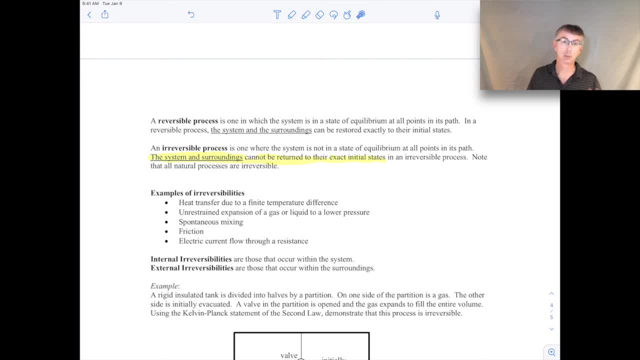 irreversible process is an idealization, even though real processes are irreversible. it's still helpful to think about reversible processes because, again, they serve as an idealization kind of the perfect case, and then that serves as a benchmark that we can compare against so we can take real processes and see how close we can get to that ideal state, and that allows us to define. 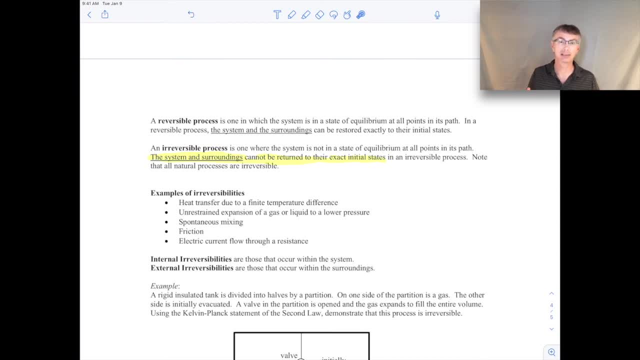 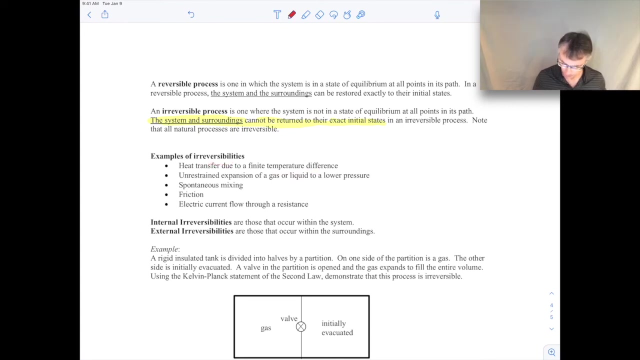 efficiencies and compare real process processes to see which ones are better than others. okay, so it's very helpful to have this idea of a reversible process now. examples of irreversibilities in nature are heat transfer due to a finite temperature difference. so let's say we had two objects here, one that's hot. let's say this one's at 100 degrees c. 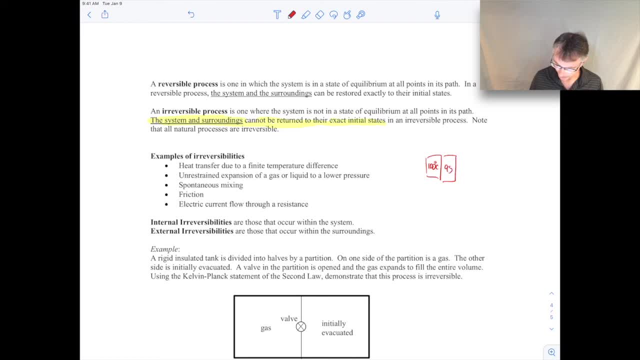 and then this one's at 95 degrees c. so there'll be some heat transfer from the hot to the cold here. that is a finite temperature difference. right from 100 degrees c to 95 degrees c. that's five degrees difference. that's a finite temperature difference. so that's a finite temperature. 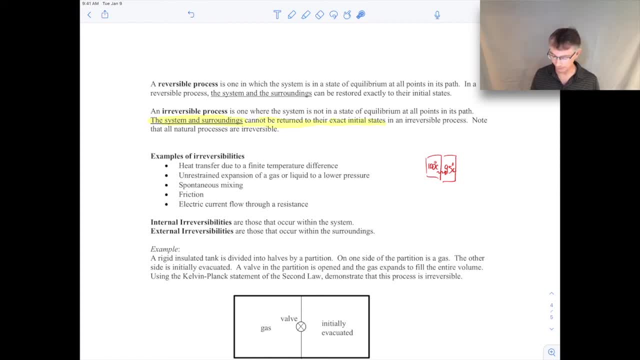 difference in temperature. and if you have that kind of finite difference in temperature, there's going to be some irreversibility occurring in that process because of the way the molecules vibrate and such, and then they, they're those vibrations kind of spread out. if you have an 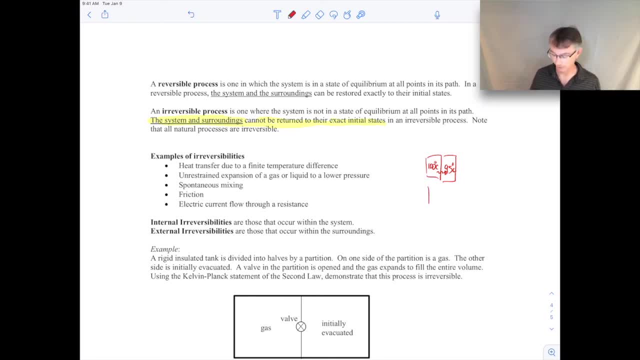 infinitesimally small temperature difference, then it becomes increasingly reversible. so what i mean by that is if this one's a hundred and then the other object is ninety, nine point nine, nine, nine, and you know, just kind of go out for some length here, then there'll still be some heat transfer. 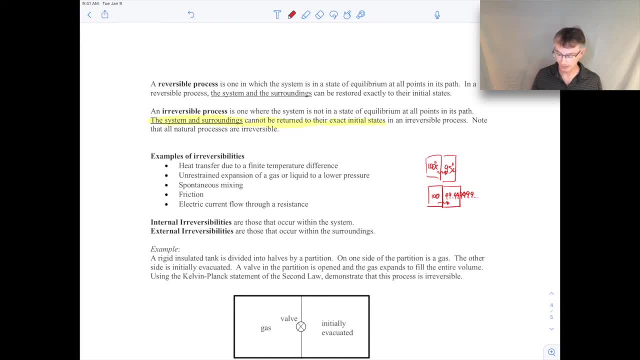 it'll be a small amount of heat transfer because there's not much of a temperature difference. but this difference in temperatures is very, very small. it's still. it's approaching a differentially small temperature. rather than being a finite temperature difference, it becomes an infinitesimally. 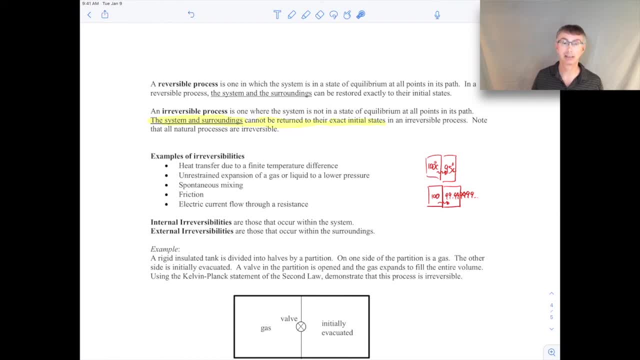 small temperature difference and so it becomes increasingly reversible. and you can imagine in the limit where this 999 goes out forever. then it does in fact become reversible. so if you have very, very, very small temperature differences, it becomes closer to being reversible. big temperature differences are more and more irreversible. another example of 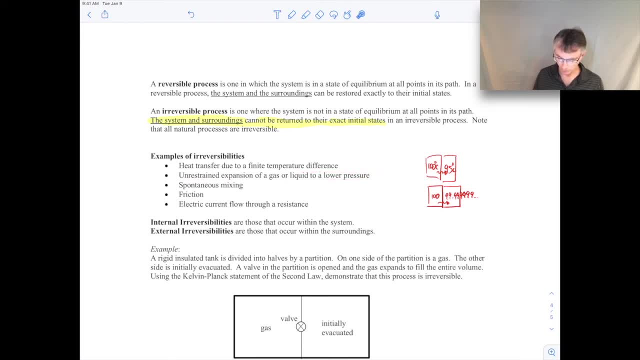 irreversibility is unrestrained expansion of a gas or liquid to a lower pressure. so that would be like suddenly filling a tank, like if you had an evacuated tank and you had a tank that had a tank and then you opened it up and all this air kind of rushed into it. that would be an 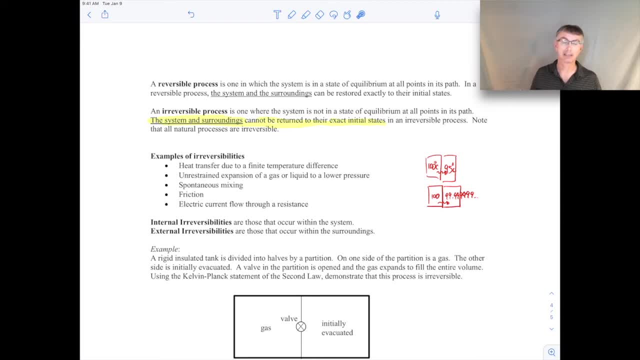 unrestrained expansion, The air would just suddenly fill that tank. That's irreversible, because we never see in nature all those air molecules suddenly leaving the tank and going to the outside right. That just never happens. Spontaneous mixing, that's like the coffee. 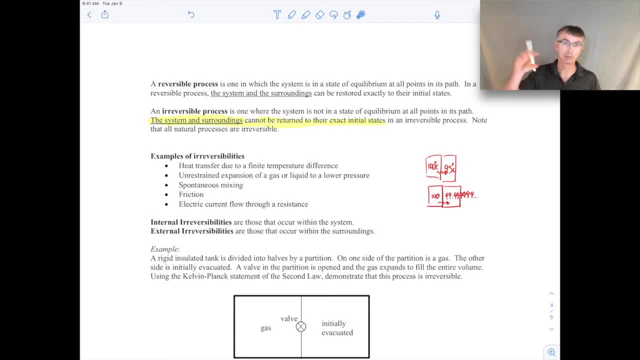 example, the cream in the coffee. It's irreversible. You can pour the cream in there and it'll, through diffusion, become more homogeneous within the coffee. You never see the reverse happening. You never see all the cream molecules suddenly coming together and forming a clump. 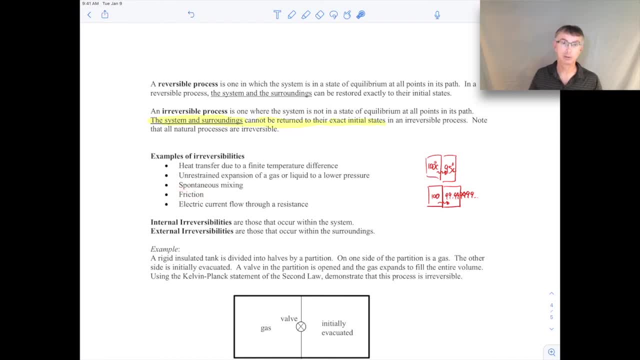 right That just that doesn't happen. Friction is irreversible. You can imagine that Friction is a dissipative process. You rub two surfaces together, energy is lost because of the vibration of the molecules involved between the surfaces, and you just don't see the molecules. 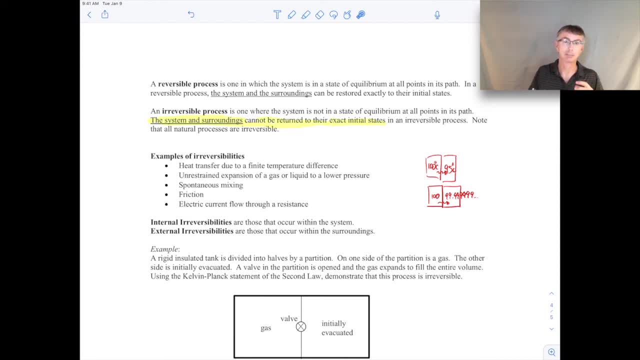 disappear On those surfaces vibrating suddenly in unison to move an object Spontaneously. so that that doesn't occur, Electric current flow through a resistance is also irreversible, Because again we dissipate some energy, the heat- and that you don't suddenly see all the molecules coming together, turning into electricity. 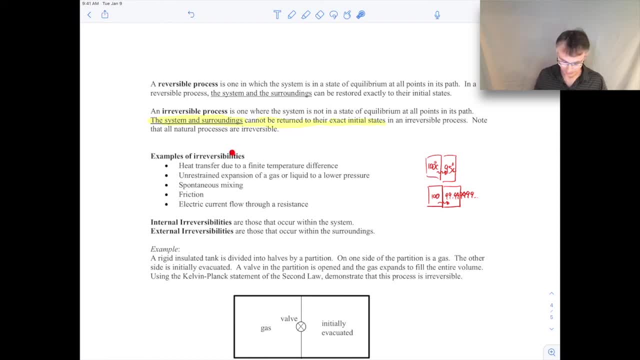 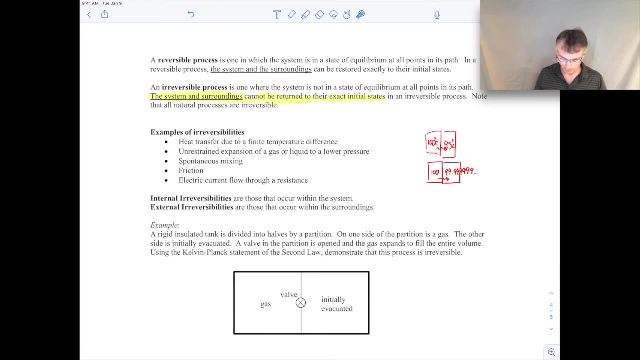 It just doesn't happen. So these are all examples of irreversibilities, and there are other examples out there as well. Internal Rear irreversibilities are those that occur within the system and external irreversibilities occur within the surrounding, so it will Refer to internal and external irreversibilities throughout our discussions. 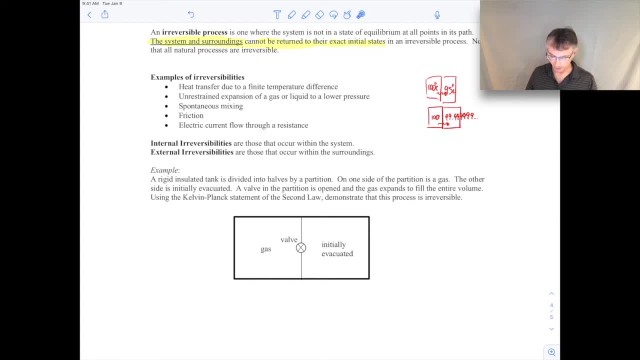 So let's do an example proving that a particular process is irreversible, And so the example is this one: we have a rigid insulated tank And it's divided into halves by a partition- So you can see the partitions right here- and we have this valve and the gas is all originally on one side, and 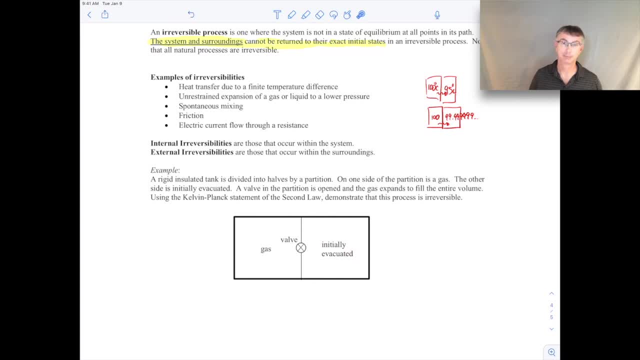 Then it's initially evacuated over on the other side. Okay, and what we're going to do is we're going to open that valve and the gas will rush from one side to the other, And we're going to just prove that we can't do the opposite. 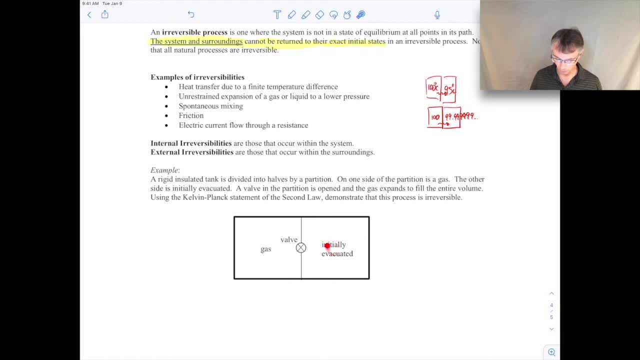 We can't have if there's gas on both sides but we won't be able to have the gas going from one side all the way back into the other, because that that would. We'll show that that will be a violation of the Kelvin-Planck statement, of the second law. 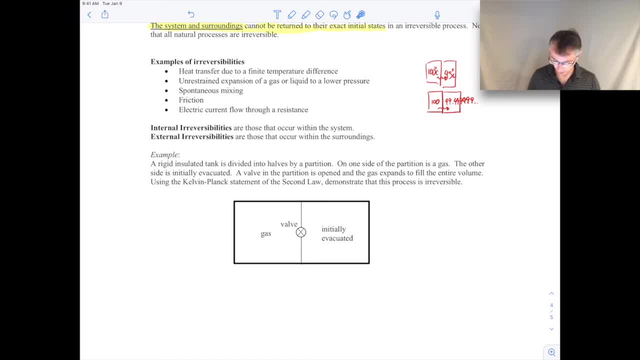 so let's first assume that the process is actually reversible, will start initially with the gas in both sides of the container and Then we'll assume that, since the process is reversible, all the gas from the right hand side Will flow into the left hand side. so we're going to assume that that's possible. okay, and that'll only occur if the process is reversible. that 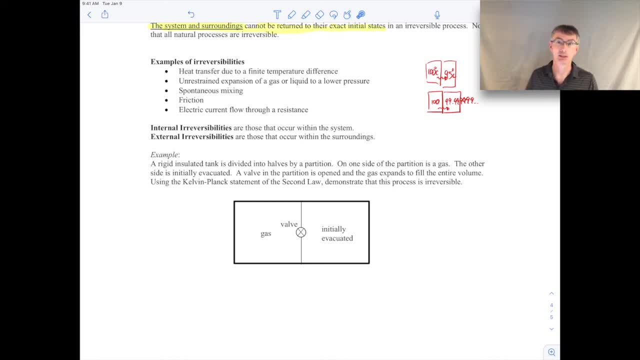 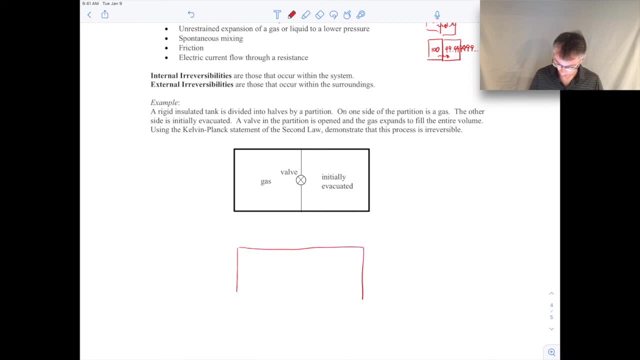 the gas can spontaneously go from both chambers in. all the gas molecules go into one chamber. now, if we do that, let me go ahead and sketch it out down here. so what we're going to do is assume that that's possible, so that we have all the gas in here. 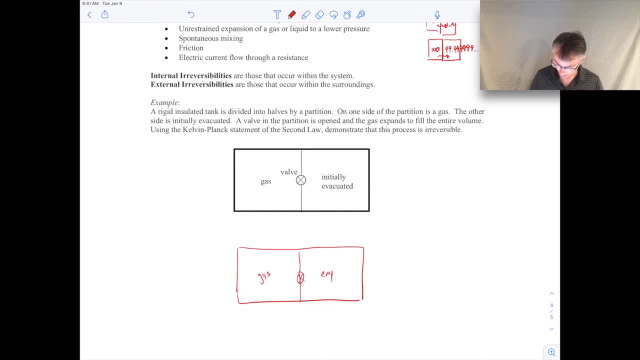 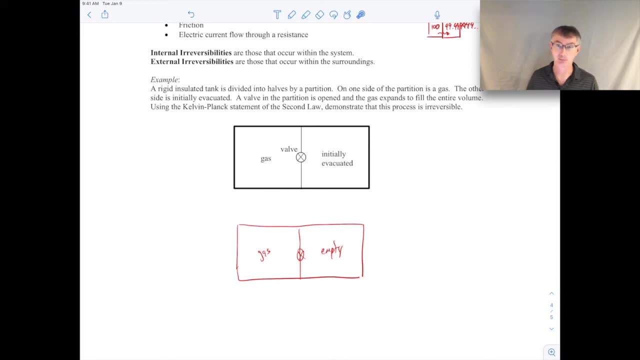 and it's gone through this valve. this is empty. when we do that, of course, that means that the pressure in this container is going to be higher than the empty part right, and what we'll do is we'll attach a turbine between the filled side and the empty side, so there'll be a turbine here. 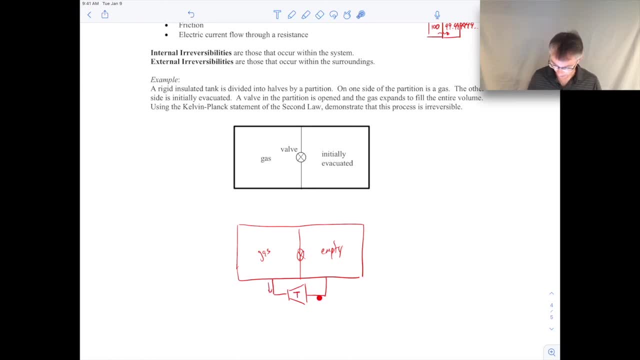 and then we'll allow the gas to flow through the turbine into the empty side until the two sides are in equilibrium and as we do that, since it's going through a turbine, we're going to extract some power coming out of it. right, there'll be some net power that we get out of that process. 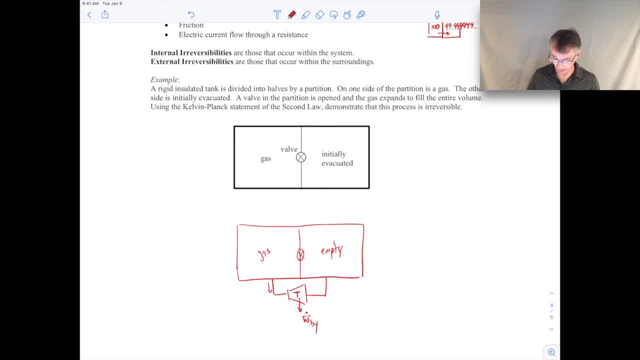 so now the system is back to where we have gas on both sides. So instead of being empty here, it'll have gas, It'll be in equilibrium. So we assume that the process was reversible, so that all the gas molecules go from one side to the other side. 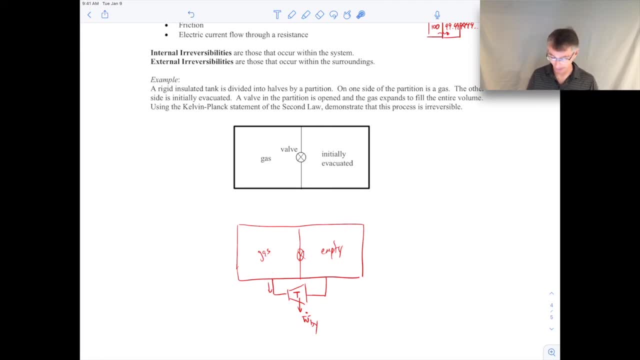 and then we'll put in the turbine and then we'll extract some power out of that. So now what we have is gas on both sides. Let me go ahead and erase this. We'll now have gas on both sides. That's in equilibrium. 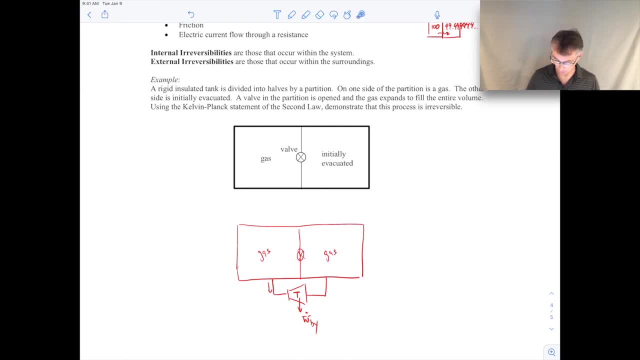 Now in the process of extracting this work from the first law, we know that if we're pulling some work out of it and the walls of the container are well insulated, then that means that the internal energy must have decreased in that process. It just comes straight from the first law applied to a control volume surrounding this whole thing. 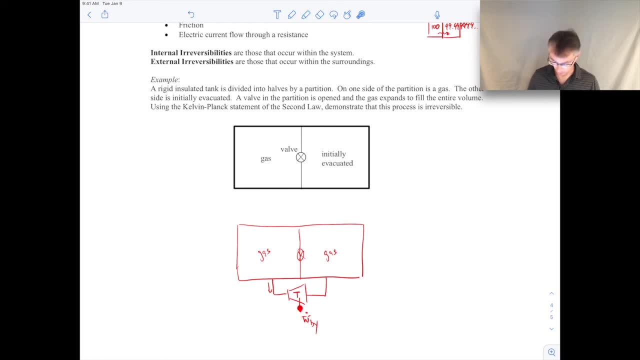 If we have no heat transfer and we pull some work out of that system, then the internal energy must have decreased. There's no change in potential or kinetic energy. So to get the system back to its original state, what we must do, then, is add some energy in. 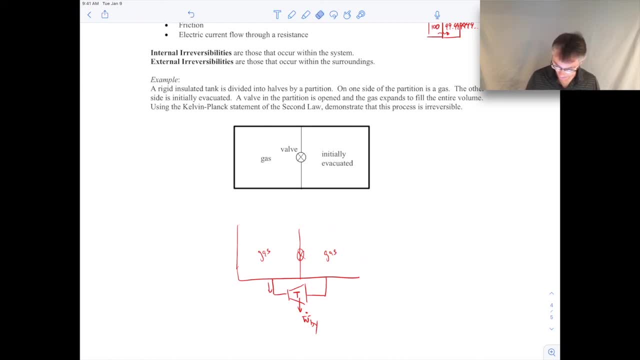 We'll do that via heat transfer. What we'll do is we'll erase part of the wall here. We'll just remove part of it and we'll put in a thermal reservoir here and then we'll have some heat transfer coming in to get us back to our original state. 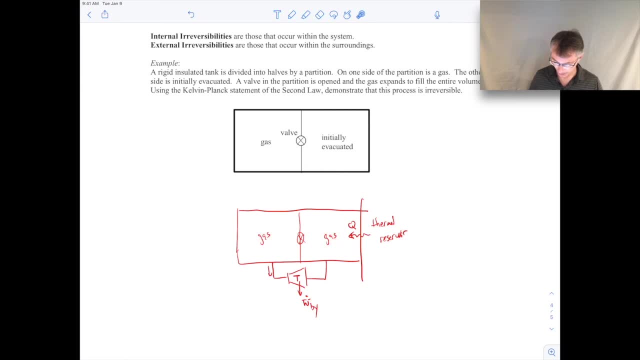 So the original state will then be with gas on both sides. since we've added some energy in via heat transfer, we'll get the gas back to its original internal energy, and then we can remove the thermal reservoir, insulate it again and go through the same process. 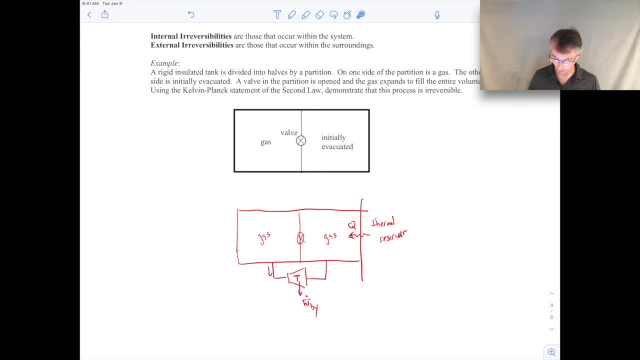 Since it's again process. one was that we're assuming it's reversible, so all this gas will go to that side. We go through the turbine, comes back in to where we have gas on both sides. the internal energy is a little bit lower. we have to get it back to its original state. 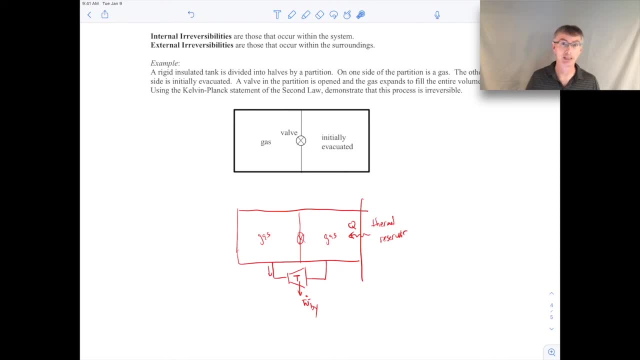 so we add in some heat and so on and so forth. So we repeat that cycle. But if you look at this for a moment, if you look at a control volume that surrounds like that, that now looks like the kelvin-plank picture, right? 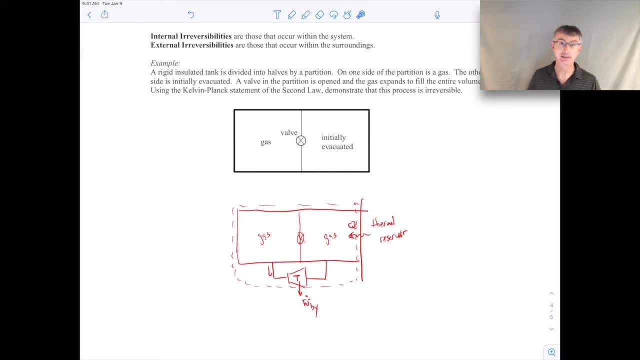 We've got a single thermal reservoir that's adding heat or energy into our system and we're extracting power from it. So we're getting positive power out of our system using a single охeter thermal reservoir and we know that's a violation of the second law of thermodynamics. So that can't. 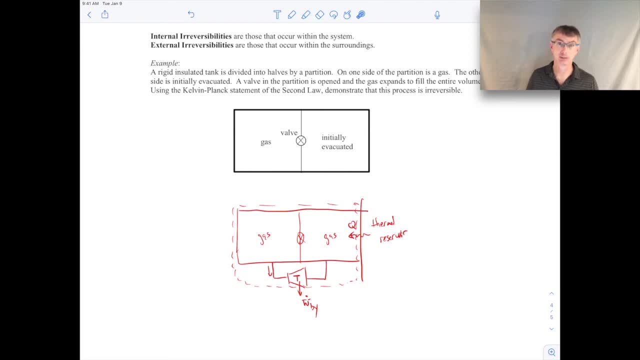 possibly happen. So something must be incorrect in our set of processes here. So let's think about what could be incorrect. Adding energy in from a thermal reservoir: well, that's fine, You can do that, As long as this thermal reservoir has a higher temperature than the gas, then we can have. 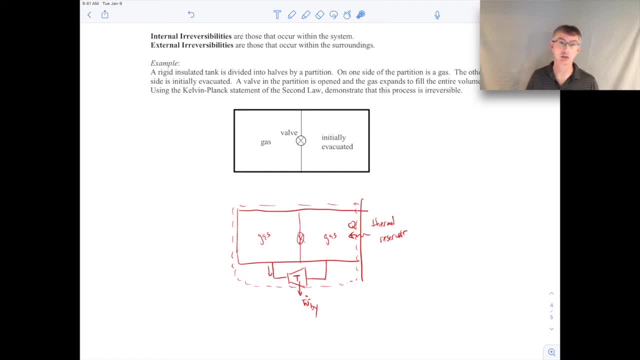 heat transfer. That's not a violation of anything. It doesn't violate the Clausius statement, for example, because we're going from a high temperature to a lower temperature, That's perfectly fine. That occurs spontaneously, So that part's okay. Pulling energy out through a turbine: 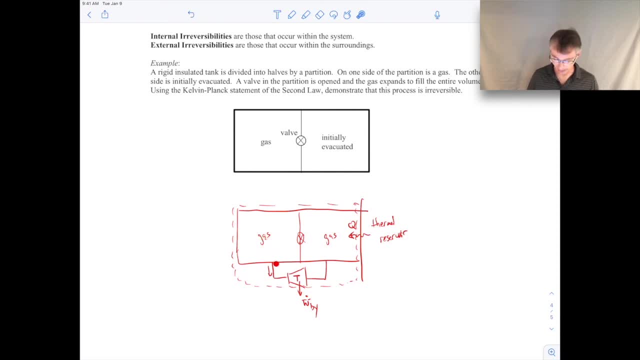 is perfectly fine. We're going from you know high pressure gas through a turbine into low- you know low pressure or evacuated container. We can do that. That's no problem either. So that process is okay. The one process then that's left is where we go from gas on both sides. 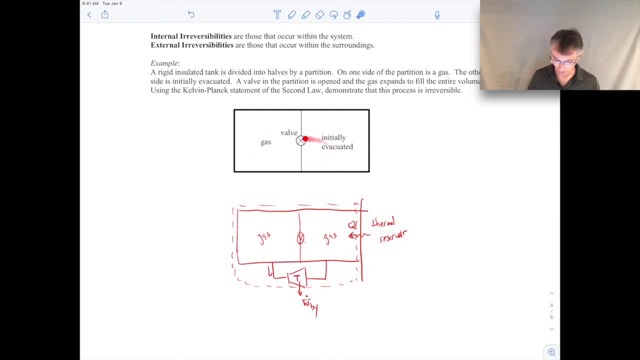 to suddenly All the gas being on one side, kind of like the picture up here, where it's evacuated and gas is all there, That very first process where all the gas goes from one side to the other side, that must be the process that's violated, And we said that that only occurs if it's reversible. 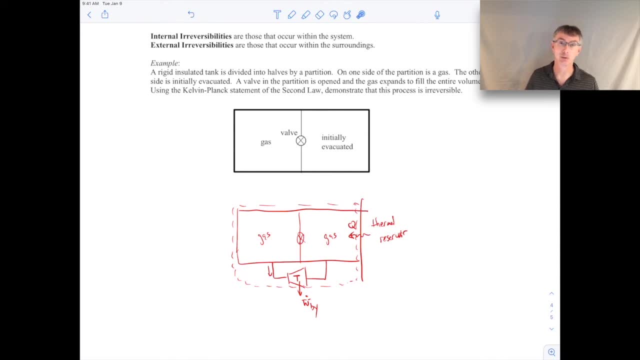 So, since we're violating the second law, the only process we could really argue that's incorrect, or the only assumption that we made that was incorrect, was that we assumed that the gas expanding into an empty container is reversible, meaning that all the gas could go back into one. 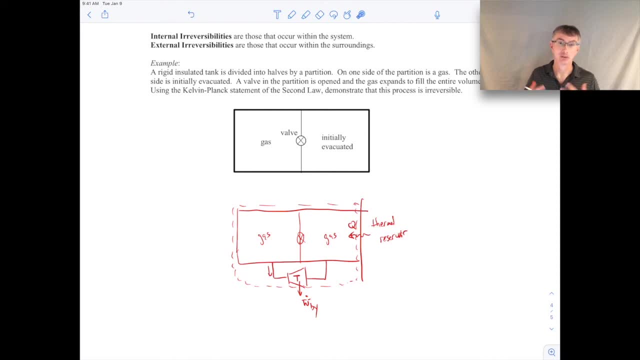 container. So that's not a violation of anything. So that's not a violation of anything. That must be the incorrect assumption. So that process of gas expanding into a container must actually be irreversible. Okay, so hopefully you follow the logic there. You have to kind of think. 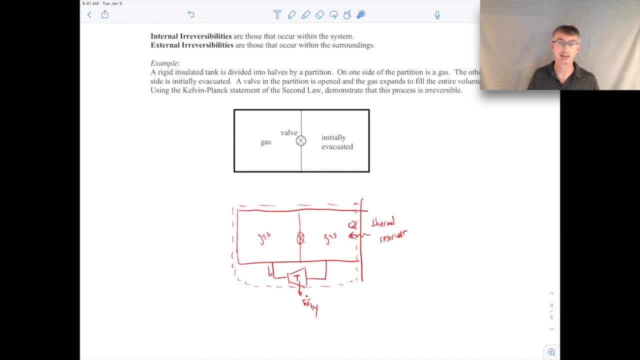 your way through it. We just showed, by using the second law, that gas expanding into a container has to be an irreversible process, because if it was reversible then we would be able to violate the second law of thermodynamics in this example. Okay, so that's an example of how we can do that. 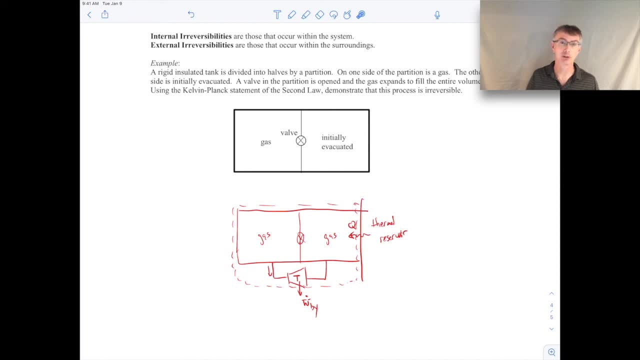 How we can show that certain processes are irreversible versus reversible by using the second law. We don't do this very much in practice, but it's worthwhile to see at least one example of it, just to show how these thought experiments can be useful. Okay, well, let's move on. 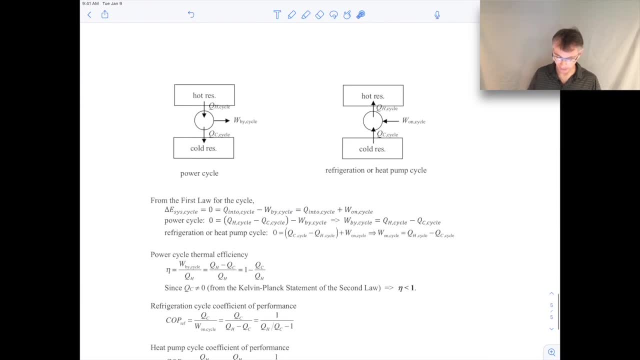 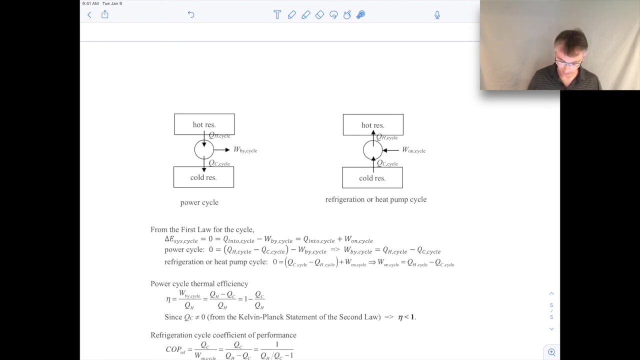 I want to talk about some of the implications of our second law statements and how that affects the thermal efficiency and coefficients of performance that we talked about in prior examples. So, if you recall, we had our schematic for a power cycle, shown here on the left-hand side. 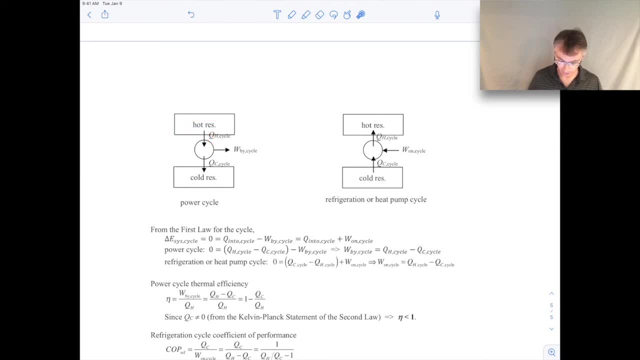 where we have a hot reservoir that brings in energy- QH- into our system and then we offload some energy, the QC, into a cold reservoir and we get some power or work out of that cycle, And then our refrigeration or heat pump cycles are shown here, where we put some power or work. 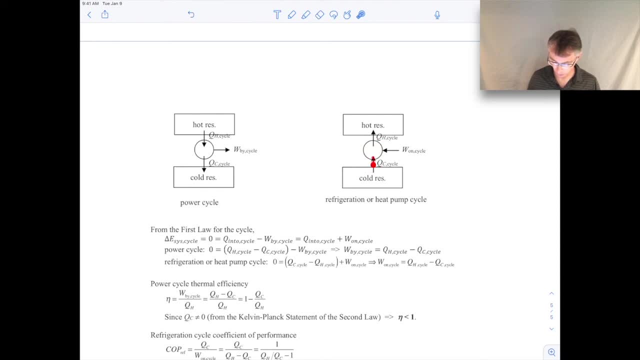 into our system and that allows us to move energy into our system. So, if you recall, we had a cold reservoir, the QC, here into a hot reservoir, QH. So we've talked about that in previous video lectures. What I'm doing right now is actually a review, but what we did is we applied. 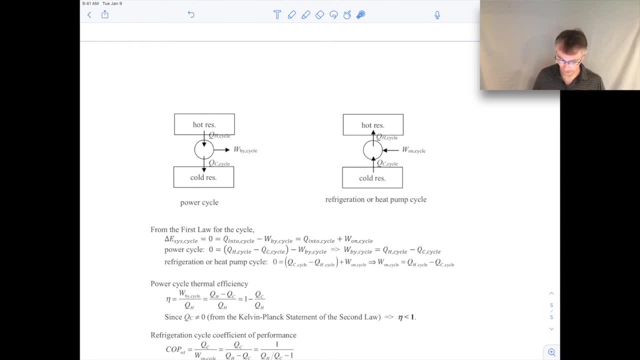 the first law for the cycle, for the power cycle for example. So we did a little control line here around our system applied the first law to that over a cycle, Of course. over a cycle the change in total energy of the system would be zero. Over a cycle that's. 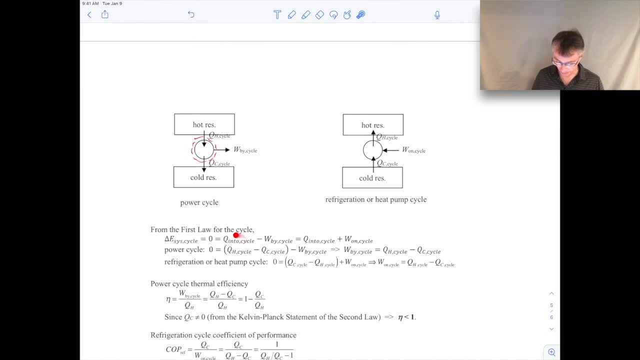 a cycle. The heat coming into the cycle in this case will be QH minus QC. so that's given right here And the work done by the cycle is right there, so that we can rearrange it to get this expression for the power cycle, And we can do a similar thing for the refrigeration. 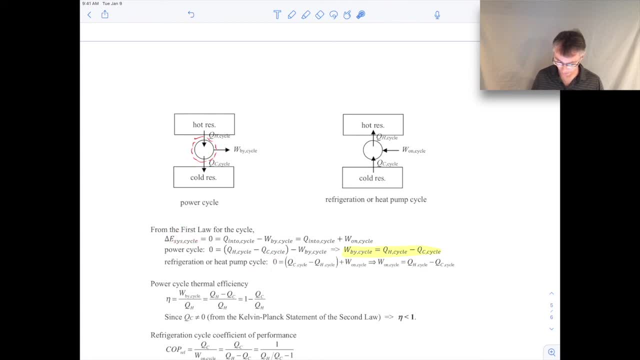 or heat pump cycle. The change in total energy of the system over the cycle is zero. The net heat coming into the system- the system here is again, this region here- is zero. So the net heat coming in in that case is going to be QC minus QH. That's right there. 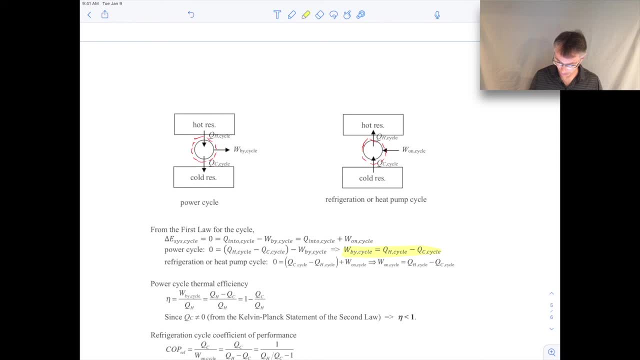 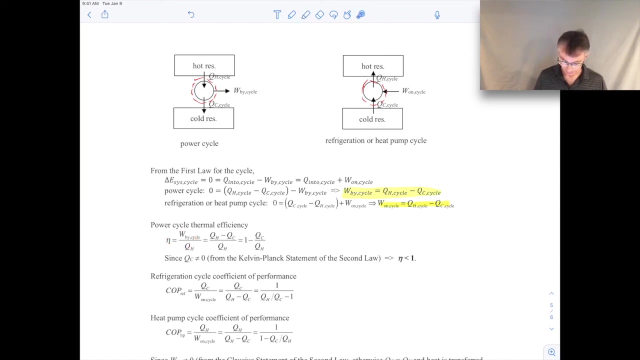 Here we have work being done on the cycle, so we have a plus W there. So then we of course get that expression from our first law analysis And then our power cycle. thermal efficiency that we defined in a previous video lecture was defined as the – so this is for the. 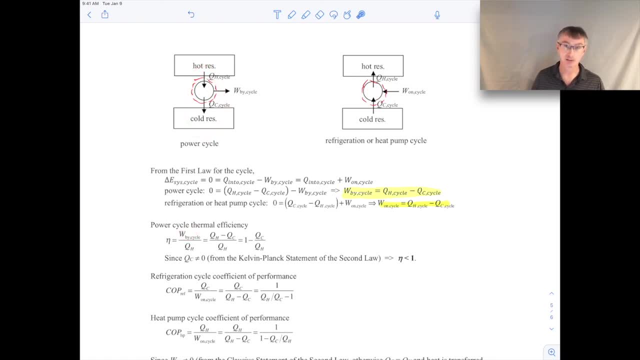 power cycle. It's the work that we get out of the cycle – that's what we want to maximize – divided by the – the heat that we have to put into the cycle – or into the system that's coming from the hot reservoir. That's our cost, So we want to maximize that The work. of course. 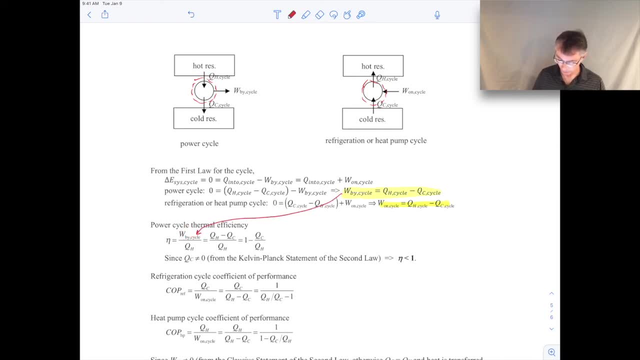 we can substitute in our expression from the first law there and we're left ultimately with that expression: 1 minus QC over QH. Now, since we have our Kelvin-Planck statement saying that it's not possible to have QC equal to zero, right, It has to not be equal. 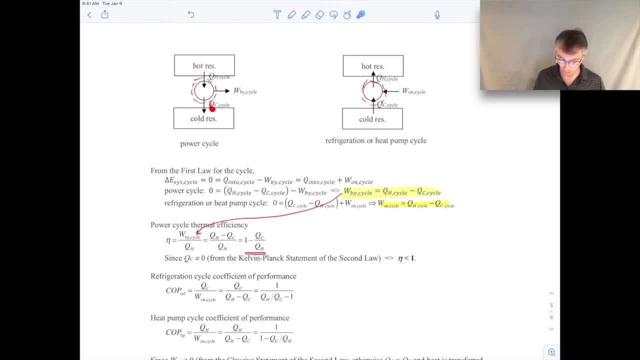 to zero, Because if it was equal to zero, if there was no QC here, then it would look like we're extracting work out of our system when we just have a single thermal reservoir, because we wouldn't have a cold reservoir because the QC would be zero. That we know is a violation. 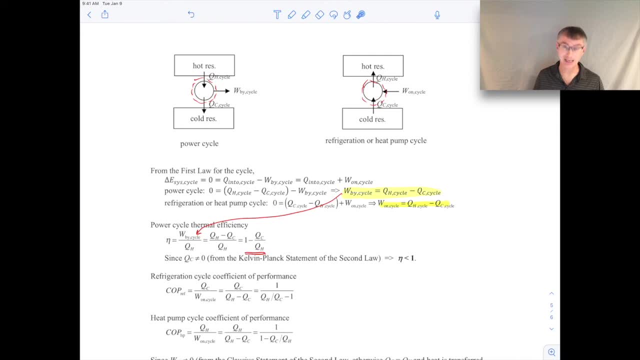 of the Kelvin-Planck statement, of the second law. so we know that QC cannot be zero. And if QC cannot be zero, then we know that the power efficiency always has to be less than 1. It can never be equal to 1.. 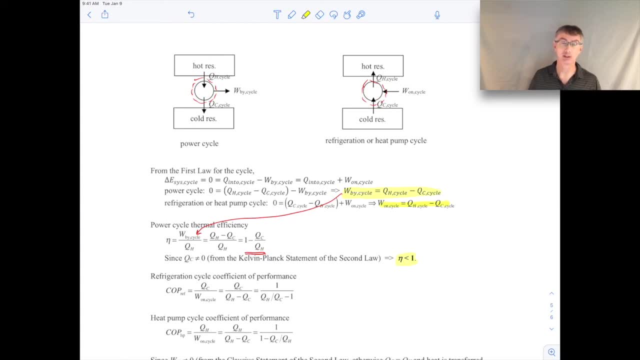 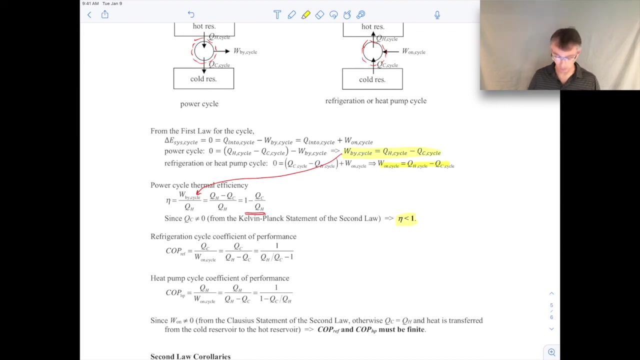 Right. So that's one implication of the second law of thermodynamics, specifically the Kelvin-Planck statement, is that the thermal efficiency for a power cycle must be less than 1, because the QC cannot equal zero. Similarly, we can make expressions for the coefficients of performance. 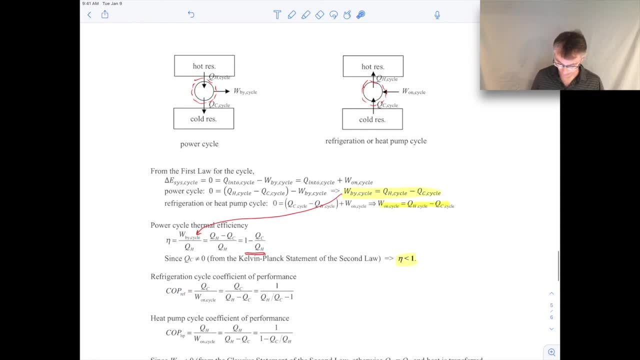 Just as a reminder, the coefficient of performance for the refrigeration cycle is QC over W into. so again, what we're trying to do is for a refrigeration cycle. we're trying to get as much energy out of the cold reservoir as possible. so the QC is what we're trying. 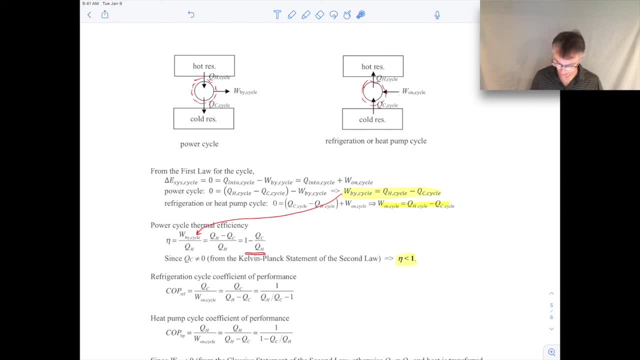 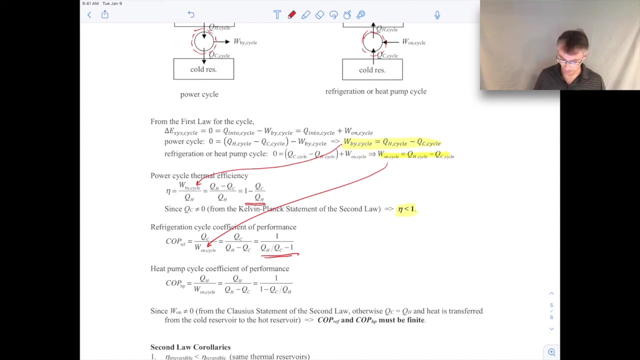 to maximize- and of course we want to minimize- how much work we have to do on the cycle. And again we can make use of the first law expression for the work, so we end up with that expression. Similarly we can do the expression for the heat pump cycle given. 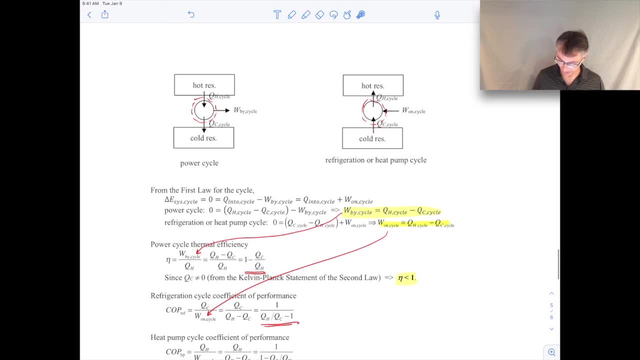 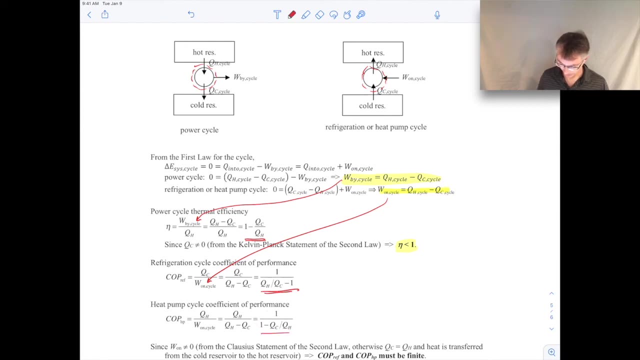 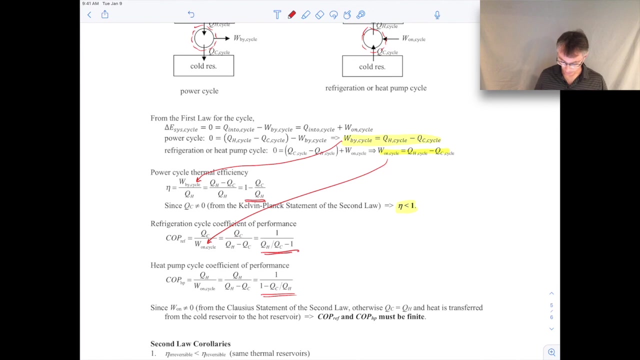 right here. There, what we're interested in doing is maximizing the heat going into the hot reservoir. So that's in the numerator here and of course we can expand that out to put it in terms of QC and QH. Now, from the Clausius statement of the second law, we know that we always have to put some 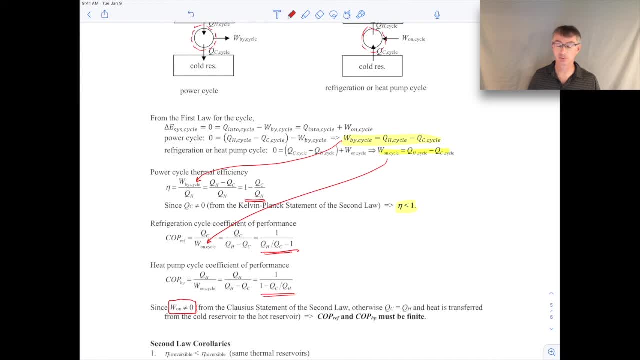 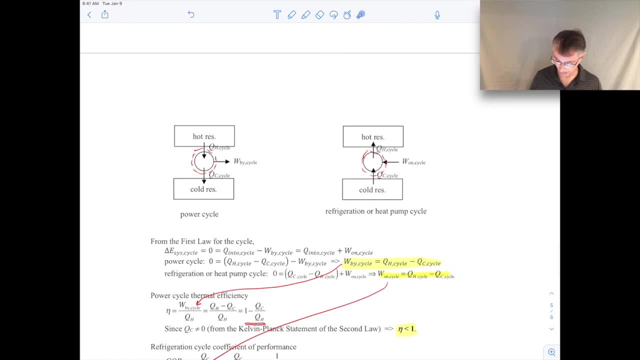 work into our refrigeration and power refrigeration and heat pump cycles in order to move that energy from the cold to the hot reservoir. so if, just looking back at this picture, we cannot have work on equal to zero, if we did have, if this was zero, then we would spontaneously be moving heat from the 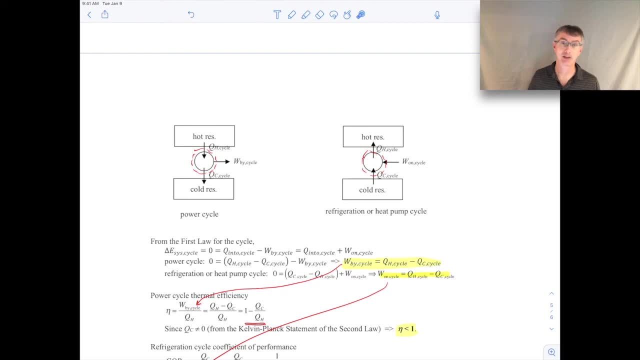 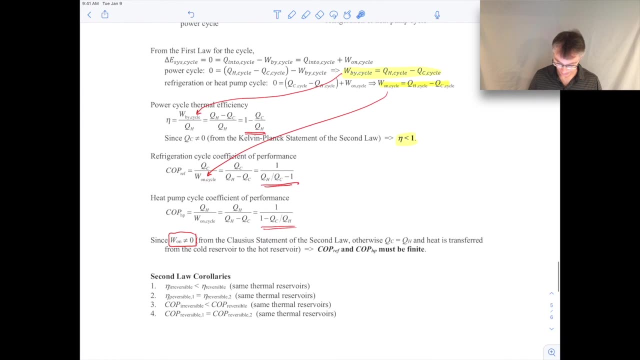 cold reservoir into the hot reservoir, and we can't have that. that's a violation of the Clausius statement. so we know that the W has to be nonzero, and if that's true, then we can see immediately, just from right here and right here, that the coefficients of performance can't be infinite, but they 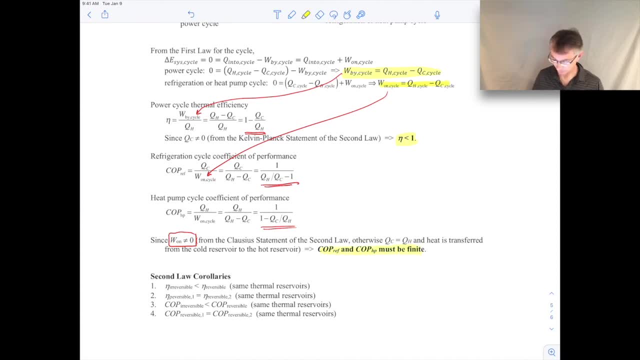 must be finite, and that's written right here. so again, making use of the second law of thermodynamics, we know that the coefficients of performance, which are measures of efficiency of heat pump and refrigeration cycles, they can't be infinite. and from the Kelvin-Planck statement of the second law, the thermal, 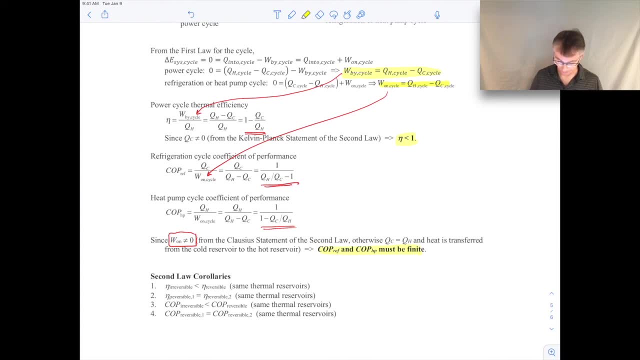 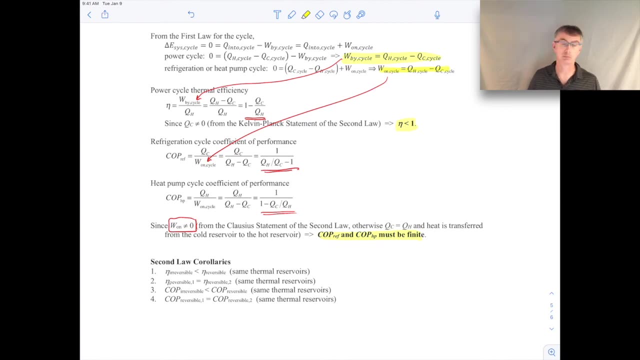 efficiency of a power cycle has to be less than one. now there's some other what we call second law corollaries that we can get from making use of the definitions of irreversible and reversible processes. I'm not going to go through the proofs of these corollaries you can take a look at. 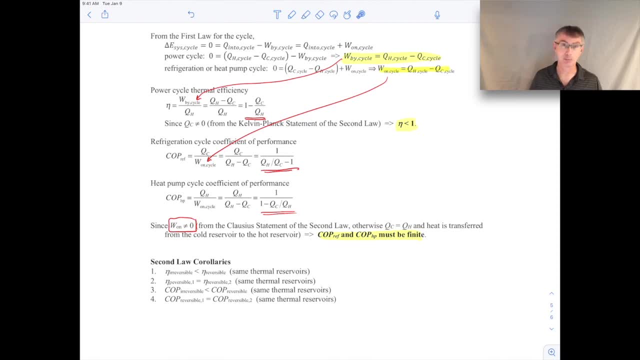 your textbook for more information on that. but I'll just state what the final results are. first, one is that the thermal efficiency of a power cycle for an irreversible set of processes will always be less than the thermal efficiency for a reversible set of processes. now, what I mean by that? 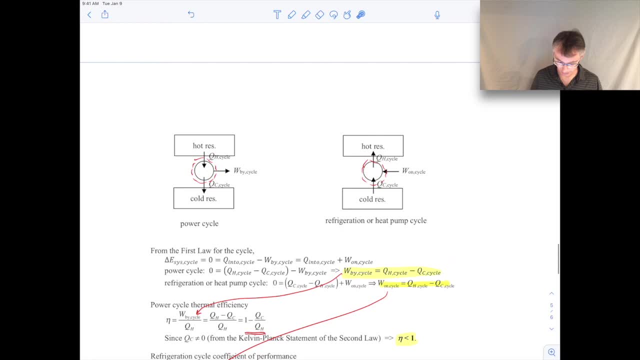 reversible. reversible versus irreversible is if you go back and look up here, remember this is our system and inside our system is where we have all of our Different devices, you know, like heat exchangers and turbines and compressors, etc. They're all contained in here. now, if those devices 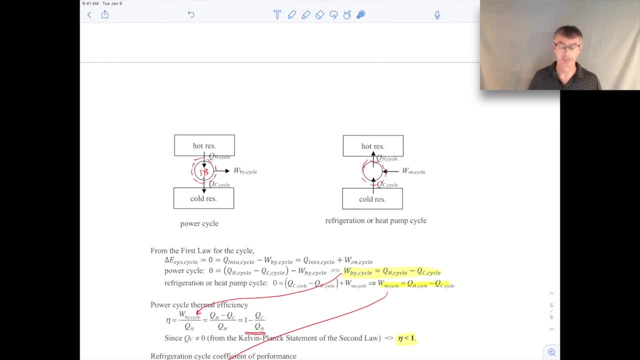 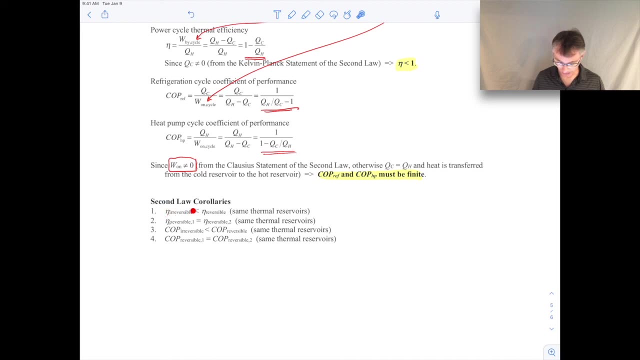 operate Irreversibly, then ultimately what we'll find is that the efficiency of that Power cycle, with those irreversible processes, it will have a smaller thermal efficiency than a set of devices that operate reversibly. so if we have Turbines and compressors and heat exchangers that are idealized and have no 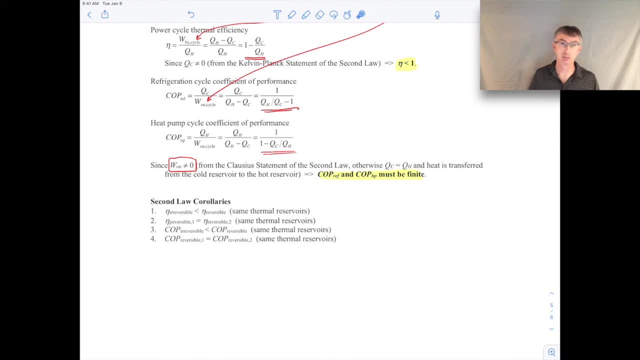 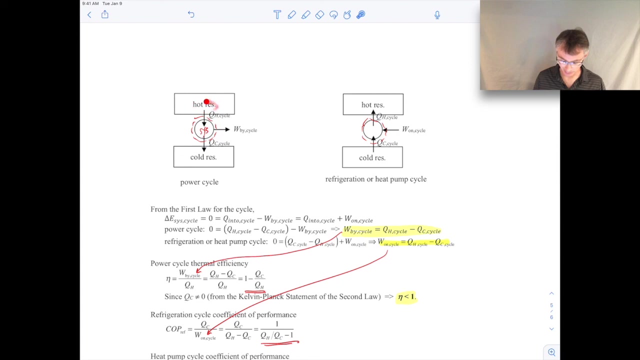 Irreversible, no irreversibilities at all to them, so that they're all perfectly reversible. then that system will have a higher thermal efficiency than one that's irreversible, assuming that they're operating between the same two thermal reservoirs, so that the Hot temperature, the hot reservoir temperature, in the cold reservoir temperature. 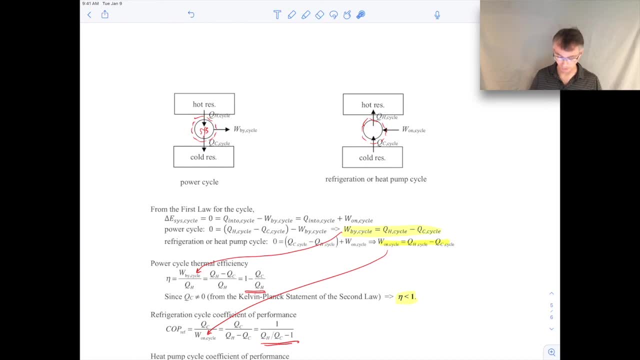 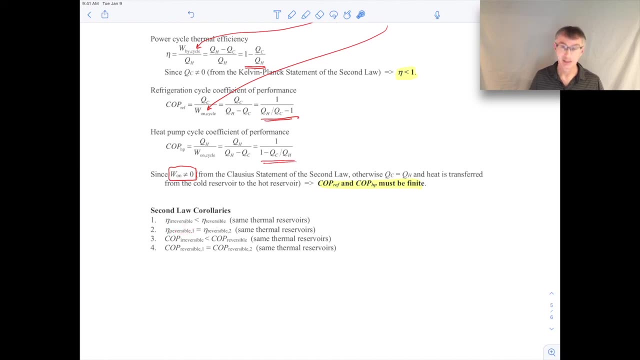 Are the same between the irreversible and reversible systems. Okay, similarly, if you have two reversible systems, Maybe they're, maybe the- the order of the compressors and turbines and heat exchangers looks a little different Within that system, but they're all reversible. So the two different kinds of systems, all reversible components, but maybe just rearranged differently, those thermal efficiencies will be equal to one another. 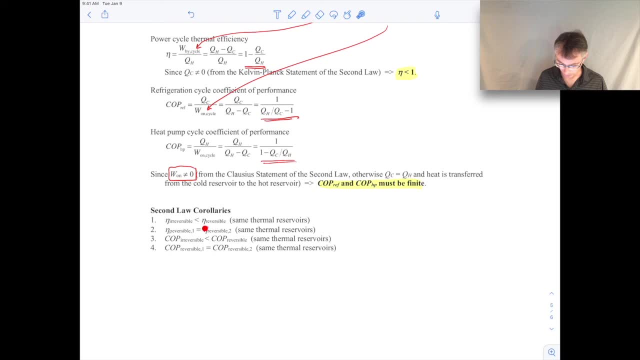 so the thermal efficiency of System one and the thermal efficiency of system two. again, if they're operating between the same thermal reservoirs, if they're all reversible, they'll have the same thermal efficiency. so it doesn't really matter what a reversible system looks like It'll it'll have the same thermal efficiency as any other reversible system. 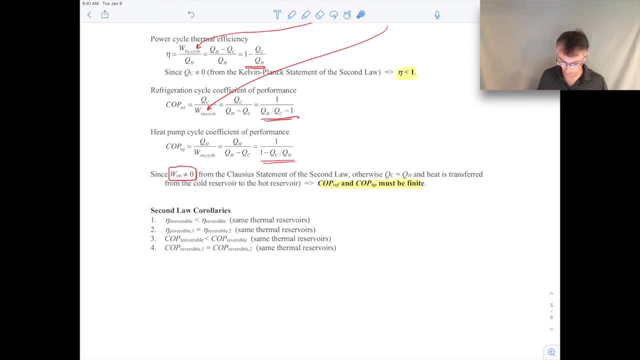 you can show the same kinds of arguments for the coefficients of performance for heat pump and refrigeration cycles: that the coefficient of performance for a system that's irreversible is less than a coefficient of performance for a system that's reversible and any to reversible systems Just rearrange the components or make them look a little different, but as long as that all those components are reversible. 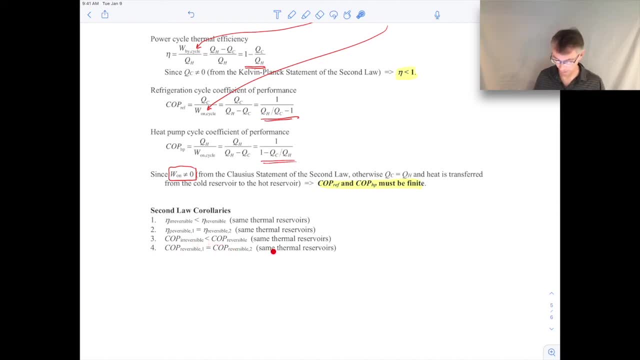 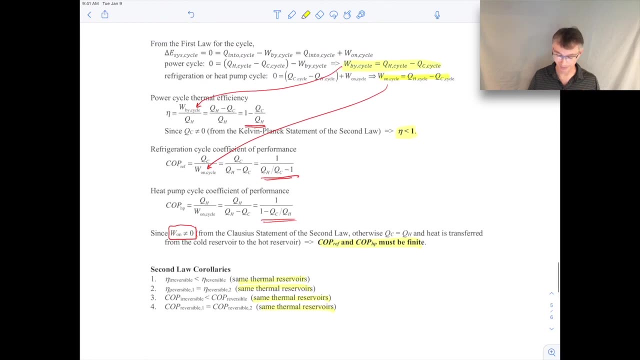 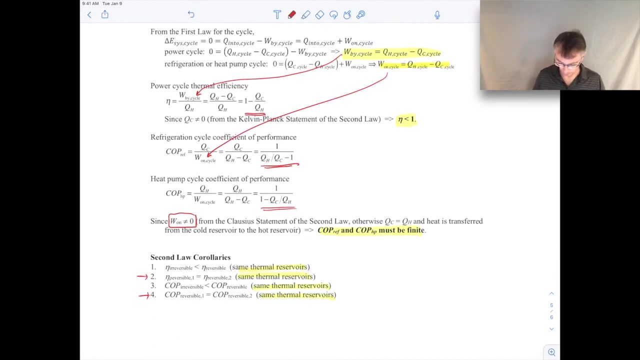 Those coefficients of performance will be the same as long as you're operating between the same thermal reservoirs the same thermal reservoir. Statements are pretty important here. They have to have this operating between the same thermal reservoirs here and Okay. so these corollaries are important, so we know that reversible systems will give. 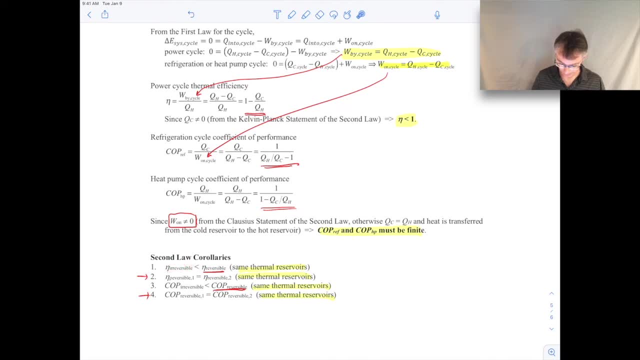 us the maximum performance, because if it's irreversible, it'll be less than the reversible case, and it doesn't matter what the reversible systems look like: they all give you the same kind of performance. So these are actually pretty important corollaries that we'll make use of. 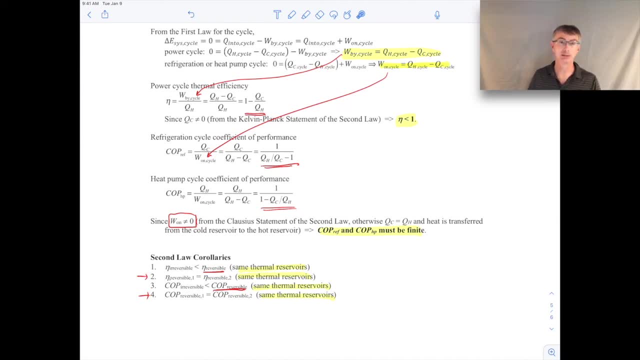 Just to recap, we talked a little bit about the Kelvin-Planck Statement of the Second Law of Thermodynamics, as well as the Clausius Statement of the Second Law of Thermodynamics. We showed that those two statements, even though they look quite different from one, 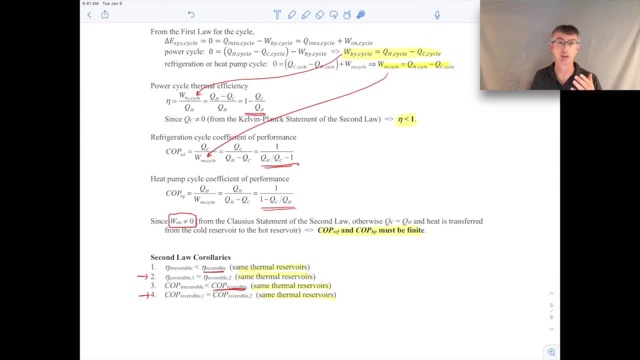 another are actually equivalent. We then also talked about what is meant by a reversible process and an irreversible process. We talked a little bit about internal irreversibility versus external irreversibility, as well as what kind of real things cause irreversibilities. 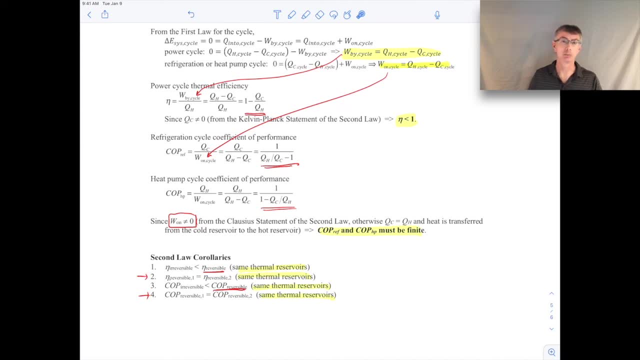 We went through a little example showing how We can prove that a process is irreversible by using the Second Law of Thermodynamics. That was the evacuated tank situation. Then we talked about some of the implications of the Second Law, namely we showed that the 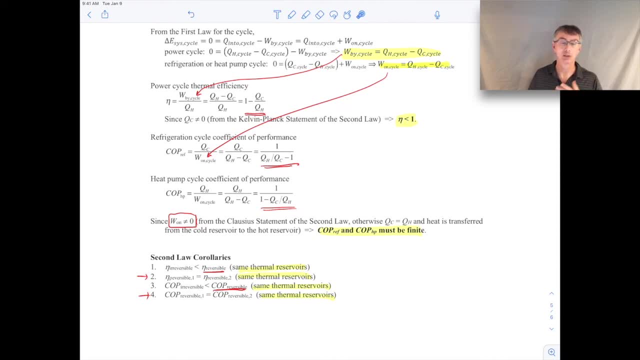 thermal efficiency for a power cycle always has to be less than one, coefficients of performance for heat pump and refrigeration cycles always have to be finite, and that reversible systems give the maximum performance as compared to, like, an irreversible system. An irreversible system won't have as high of a thermal efficiency or as high of a coefficient. 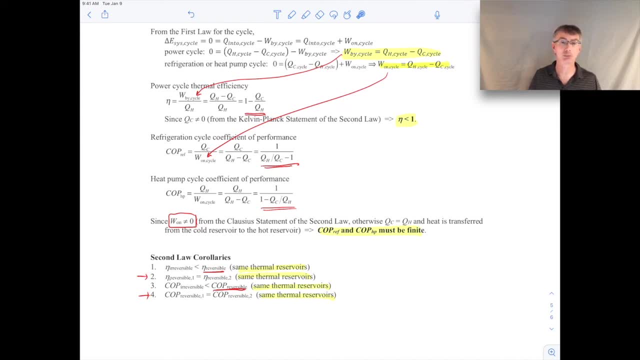 of performance and that it doesn't matter what the details of the reversible systems look like: they all give the same thermal efficiency or coefficients of performance.